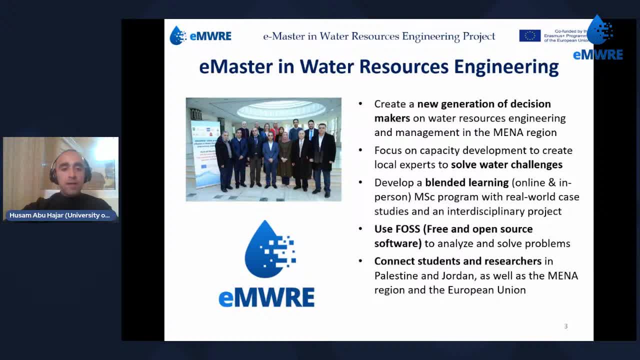 So what I'm going to be talking about today is like a brief description about our project, what we actually did and what we hope to be done over the next couple of months. So, basically, the goal of our projects or the objectives our projects are to actually create a new generation of decision makers on a very critical topic. 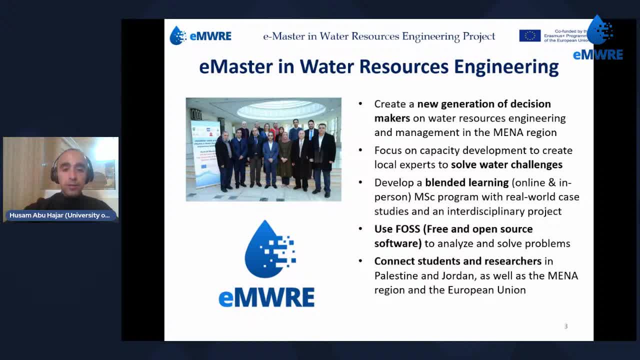 which is the water resources engineering and management in the MENA region. We are actually focusing on the capacity development in order to create local, local experts to solve the contemporary and the most challenging water water issues in our region. This is actually going to be developed by a 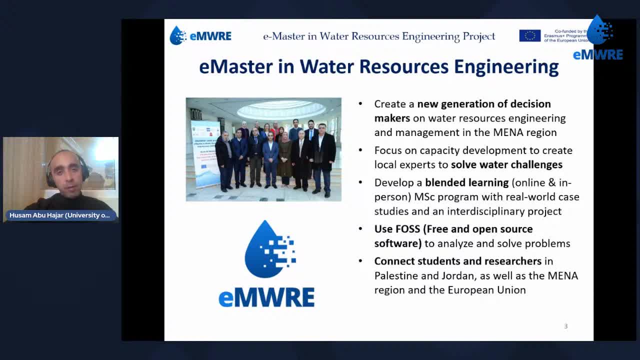 Adopting a blended learning approach. a blended learning approach where we are going to use the classic face to face teaching and class teaching, And we are also going to capitalize on the modern technology and e-learning techniques in order to actually reach an ideal combination of the two different approaches in learning. 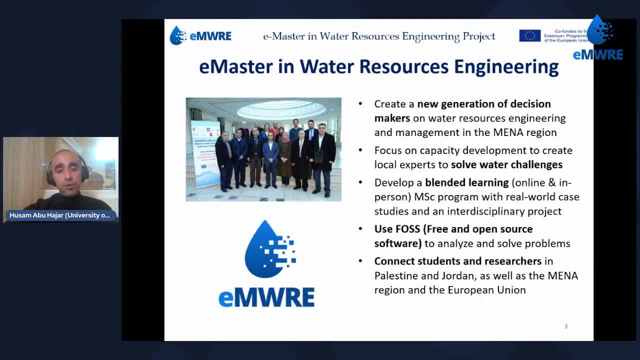 And one of the themes in our project is actually the use of free and open source software. So, if you have seen it, in our previous webinars we were only exclusive on talking about free and open software in statistics and hydrology and hydraulics and all those modeling purposes. 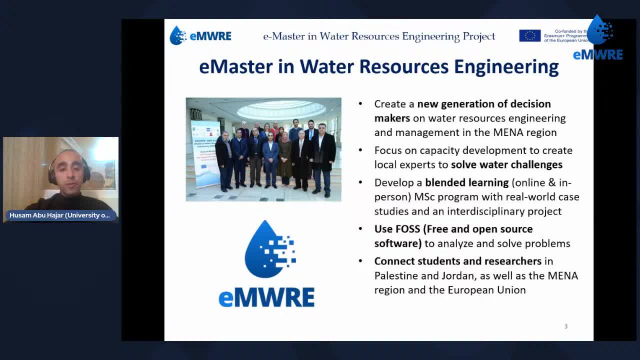 Our our project is all about using free and open source software and then finally to connect students and researchers between the two countries, Palestine and Jordan, as well as our partners and friends From Europe, ultimately to actually develop the research skills and hopefully reach or solve the problems that we face in the water sector in Jordan and Palestine. 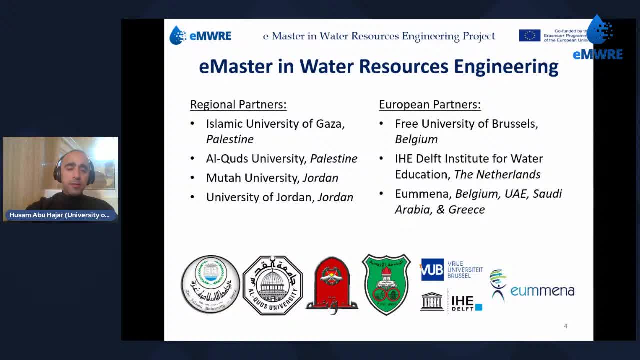 So our our partners. we have four regional partners. two of them are from Palestine and two from Jordan: the Islamic University of Gaza, Al-Quds University from Palestine, And we also have Mota University and the University of Jordan from Jordan. We also have our European partners. 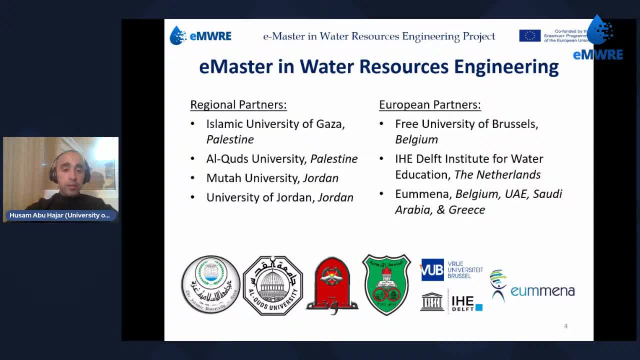 We have the University of Brussels, VUB, in Belgium. We also have the IHE Delft Institute for Water Education in the Netherlands, And we have Yumina, which is a company in Belgium. They also exist in other countries as well. 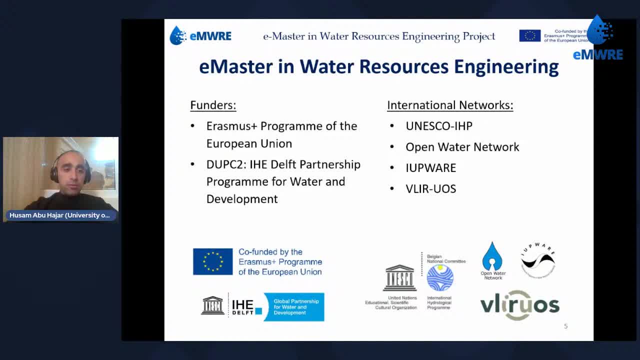 We would like also to thank our supporters. Our supporters. the program is actually co-founded And co-funded by the Erasmus Plus program of the European Union. We also have other other international international funders and European supporters. We have local supporters as well. 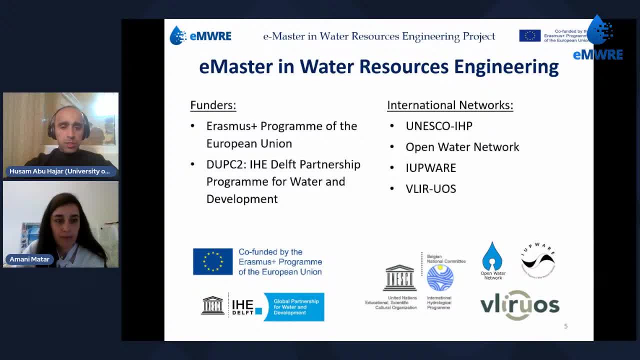 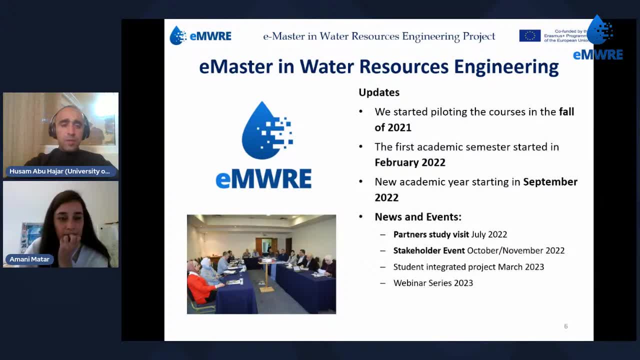 We would like all to thank you for, for the support which will actually keep our project ongoing. Next, please: Yes, So just to give you an update about our, about our ongoing activities. Next, please: We actually have started piloting the courses in the fall of 2021.. 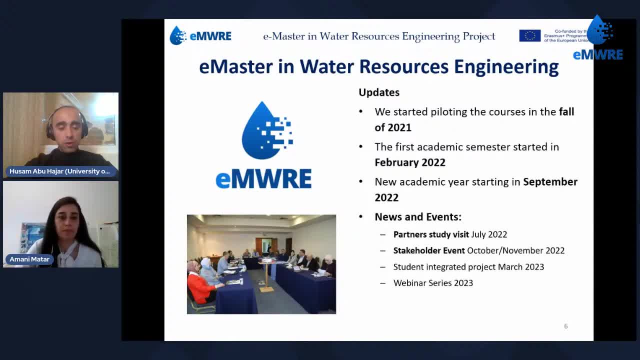 We launched three courses. These courses were exclusively online And we have we have a platform, a learning platform, where students can actually register and enroll And they will be interacting with the instructors and with the students as well In terms of the academic semesters, because the program is actually going to be launched mainly in the universities. 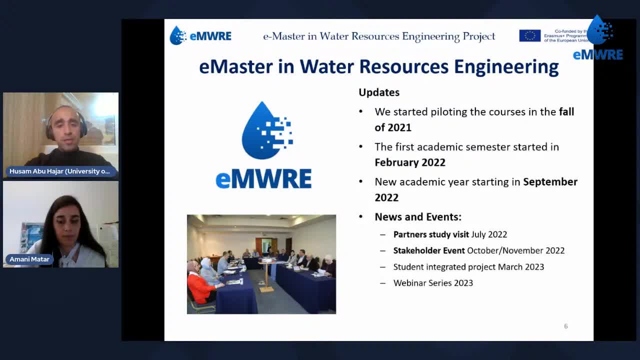 In the Palestinian universities. So the first academic year actually started in February 2022. And then the next academic year is going to start in September 2022.. These, these are some some dates for students who are actually interested in enrolling the programs and registering. 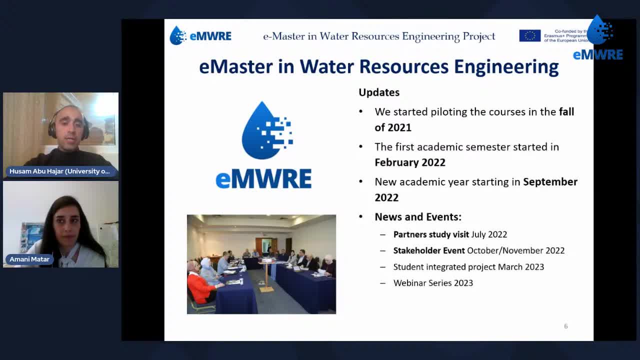 Because the key limiting factor for registration and enrolling is the registration guidelines for each, for each institution. We we actually plan to. We actually plan to conduct a partner study visit in July of 2022.. There will be a conference, we will meet and then we will work on different activities in the project. 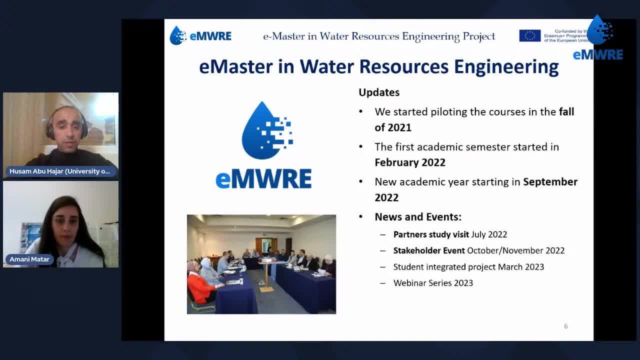 We also plan to host a stakeholder event in October or November of 2022.. We had one last year. It was. it was a success, despite the constraints by the coronavirus. It was a success. It was in Amman Jordan. We hope that we will have a bigger one. 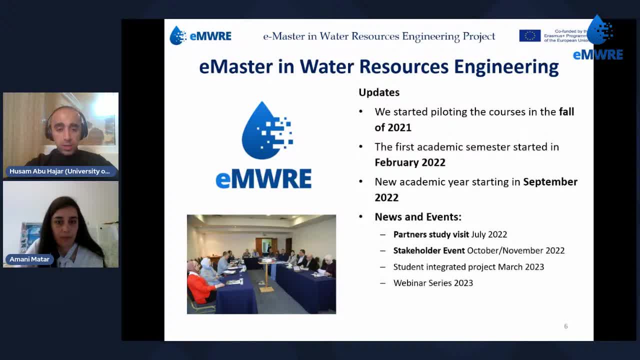 This upcoming October or November. we'll keep you posted- And then we plan to to have an integrated project for our students. The initial plan is going to be students from Palestine- They are going to have a project- and then in Jordan as well. 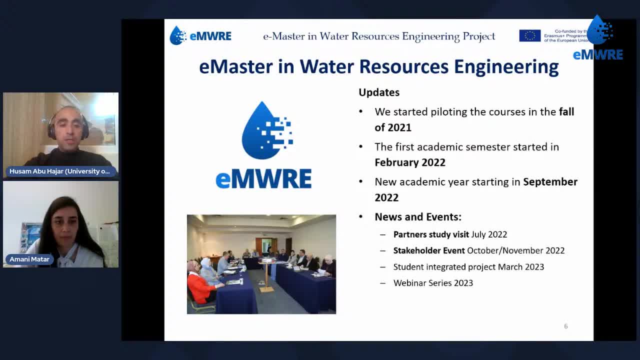 But over the next couple of months we will see what will happen. We might end up just combining the two groups together in one field study or one watershed in Jordan, And then another webinar series, And then another webinar series, And then another webinar series. 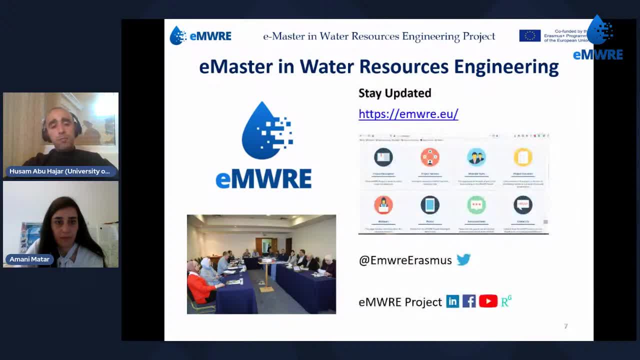 In 2023,. these activities will all be posted on our platform, Please, you can always visit our website, And we also are present on on all, all social media platforms: Facebook, LinkedIn, YouTube, ResearchGate and, of course, our our website. 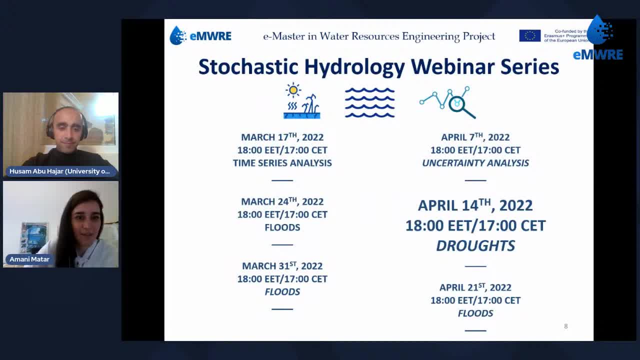 Thank you everyone And back to you, Amani. Yes, thank you very much, doctor, for this presentation And I hope you stay connected. And I hope you stay connected as well, as the doctor was mentioning, on the project website. 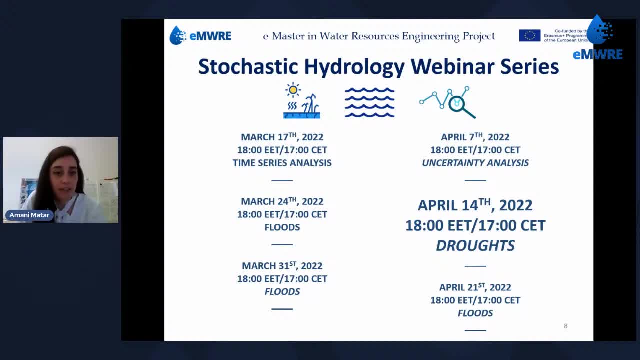 So today, as part of this project, this is the third webinar series that is being held under the project and focus on stochastic hydrology. Today we are in our fifth webinar of this series and we still have one more to go next week. 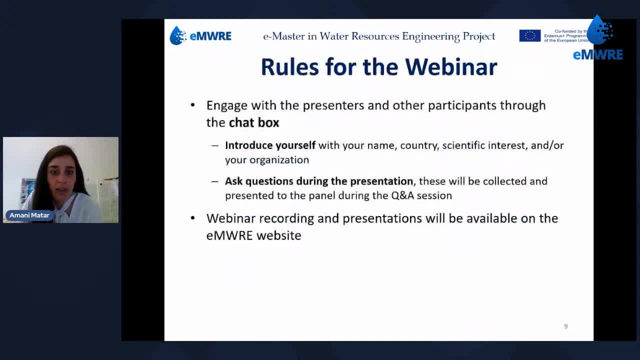 And the focus today is on droughts. a little bit of rules of the webinar. So please introduce yourself, engage in the chat box, Introduce your country, where you're from scientific interest, your organization And please ask your questions in the chat box. 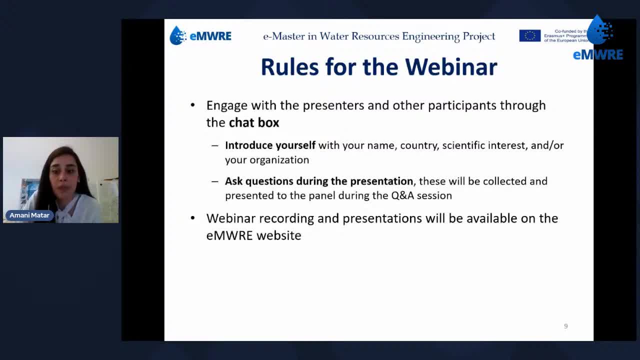 We will be addressing them at the end in the Q&A session, So just put your questions and we'll address them in the end. And the final note: this webinar is recorded and will be available on our YouTube channel on the project YouTube channel. 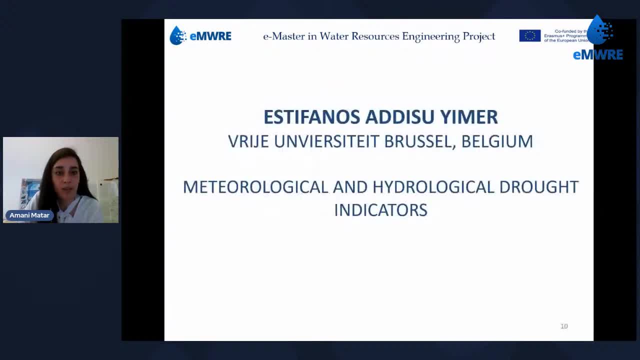 So it will be also available after to you. So today we have with us Stephanos. So today we have with us Stephanos. He's a PhD researcher from the Free University of Brussels in Belgium. He has a master's degree in water resources engineering and advanced master's in integrated nature-based solutions and technologies. 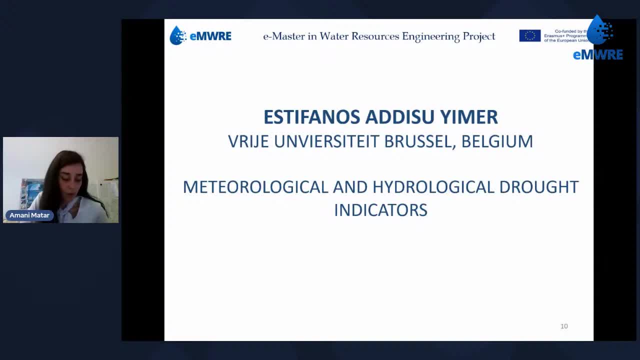 He has a strong interest in groundwater and surface water modeling and drought analysis using drought indicators. So we would like to welcome with us Stephanos, And thank you very much for being with us. Thank you, And the floor is yours. Thank you so much, Amani. 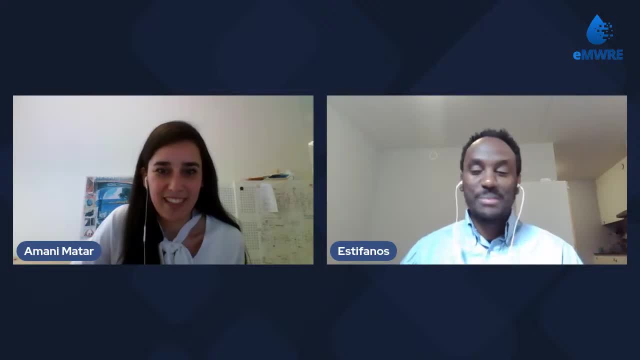 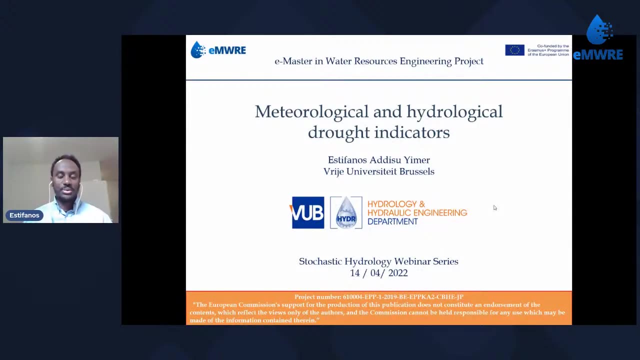 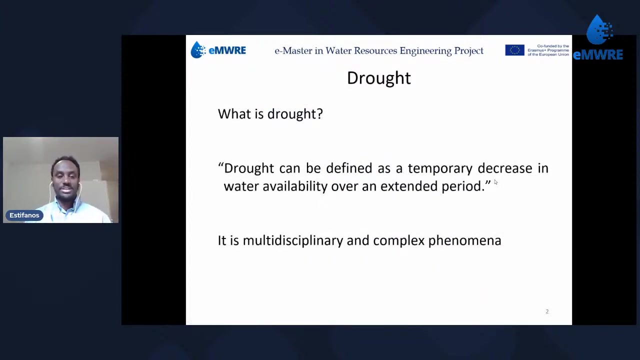 You have introduced me very well, So I will just jump into the presentation that I will discuss today. So it's about meteorological and hydrological drought indicators. So first let's start with the basic question: What is drought? Drought can be defined as it's a temporary decrease in water availability for an extended period of time. 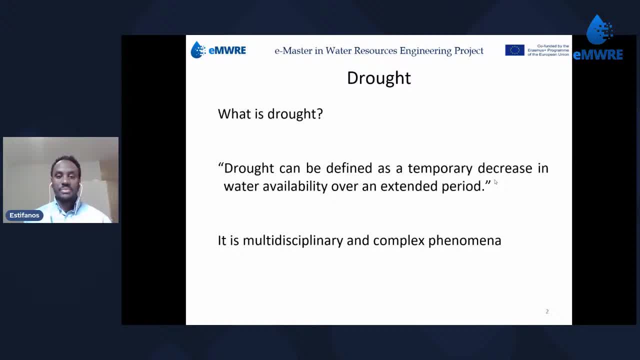 It's a multidisciplinary And a very complex phenomena. Its complexity relies on the uncertainty to predict it, Because you never know when will it happen. But there is, of course, early warning systems, But it's with uncertainty, So it's very complex phenomena. 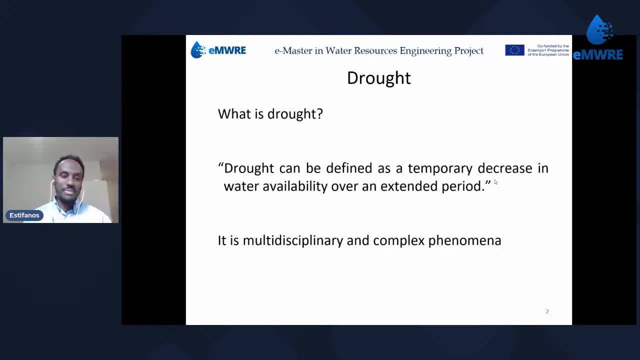 And it's also very multidisciplinary. in a sense It affects the ecosystem services, It affects the socioeconomic interaction. Also it affects the hydrological bodies. Therefore, it's a very multidisciplinary and a very interesting study area. I hope you'll enjoy it. 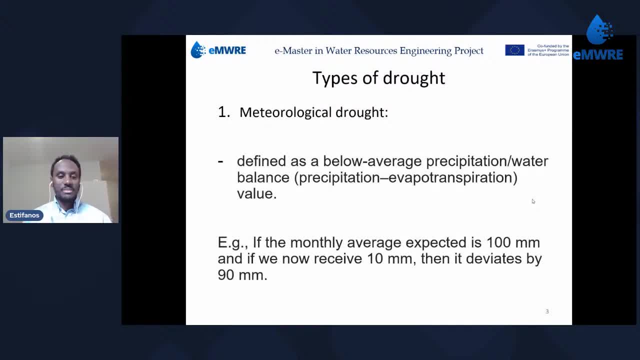 So let's start with the different types of droughts. First, meteorological droughts. These droughts, they are defined by below average precipitation or water balance value. Here, when I say water balance value, what I meant is precipitation minus evapotranspiration values. 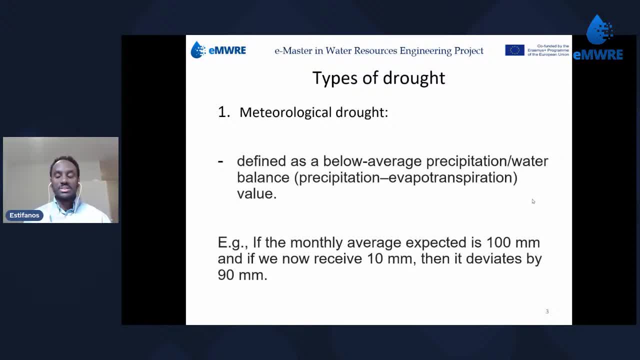 Here it's different from hydrological modeling, wherein water balance is composed of different compounds. But here, for drought analysis, precipitation minus evapotranspiration data can be sufficient, For example, if you usually expect using 30 years of historical data- usually we use 30 years of data to assess these climatic variabilities. 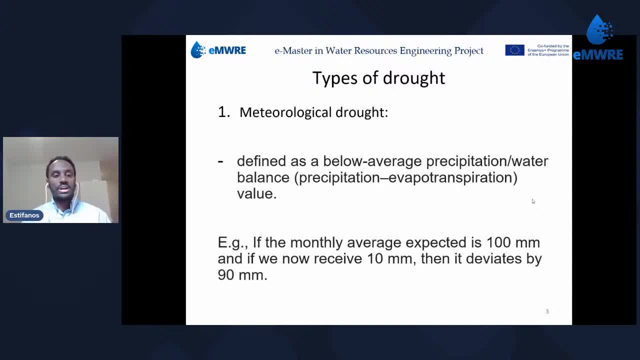 So if you expect that the average condition is 100 millimeter, but now you are receiving, let's say, 10 millimeter, it divides by 90 millimeter. Therefore, due to that, we call this meteorological drought. Okay. 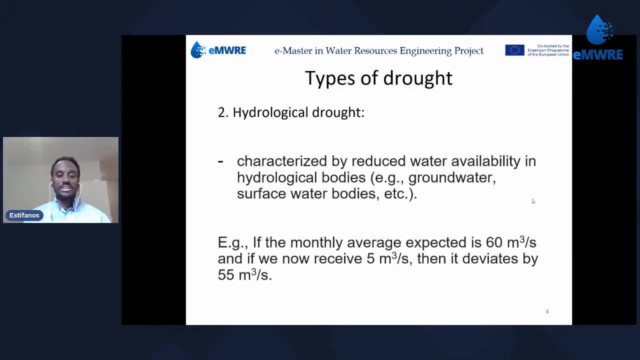 And the second type is hydrological drought, where it's characterized by reduced water availability in water bodies, For instance in groundwater bodies, surface water bodies or reservoirs in the dam levels. Is it decreasing or increasing That one? it's assessed using different indicators and we call it hydrological drought. 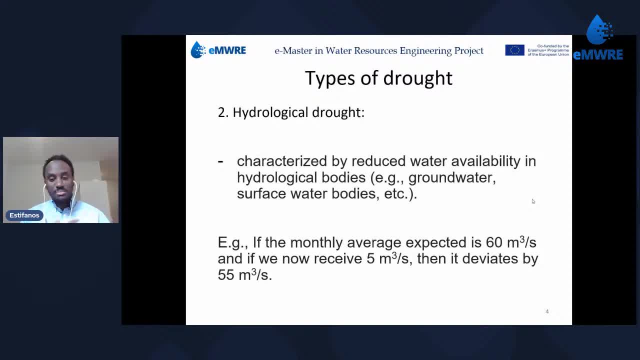 For example, in a river. let's say you expect, based on, as I explained, 30 years of data, let's say 60 metric cubic per second of stream flow, But now you are receiving 5 metric cubic per second. 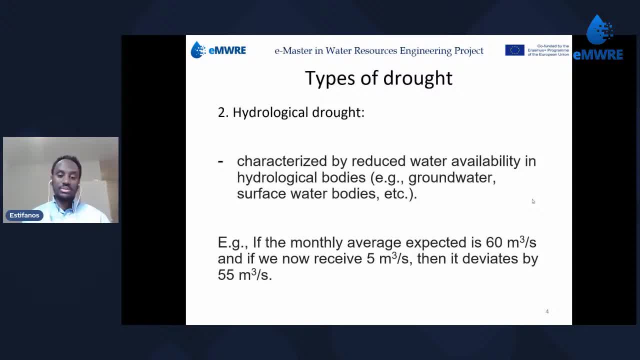 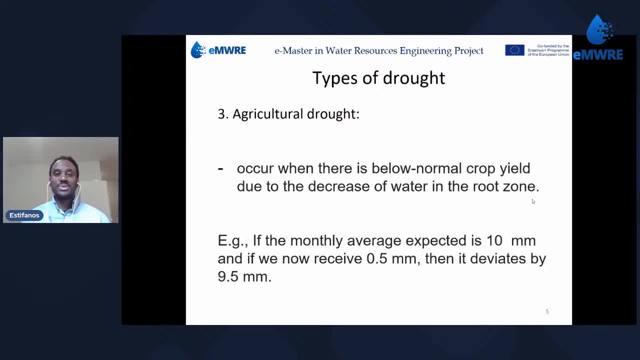 Then it substantially deviates from that normal condition And that we call it hydrological drought And we have also agricultural drought. This is a very important one, because we have to eat to survive, And this affects the agriculture sector. That is, if you are experiencing below average soil moisture in the root zones, then the crops will wilt or they will desiccate. 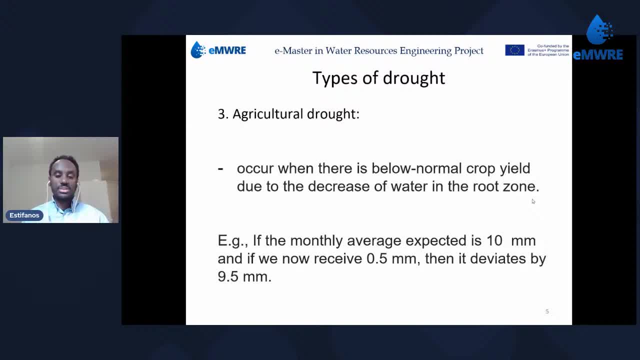 Due to that, agricultural drought can happen, For instance, usually in the root zone. if we expect 10 millimeter of soil, let's say 10 millimeter per millimeter, let's say: And if we are receiving now 0.5, then it deviates a lot. 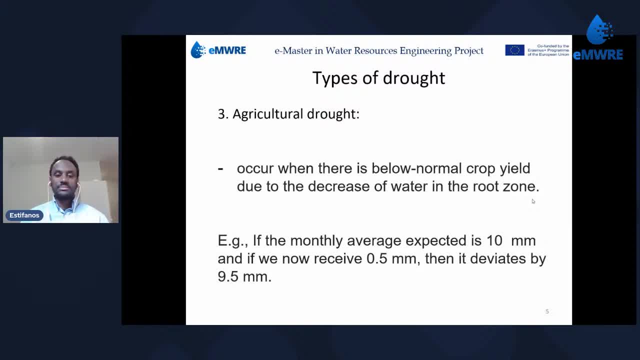 Therefore, due to that, we call it agricultural drought, But there are also socioeconomic droughts. This is what we call the aftermath of drought. That is, for instance, if our water supply is not able to be met by the water resource systems that are available. 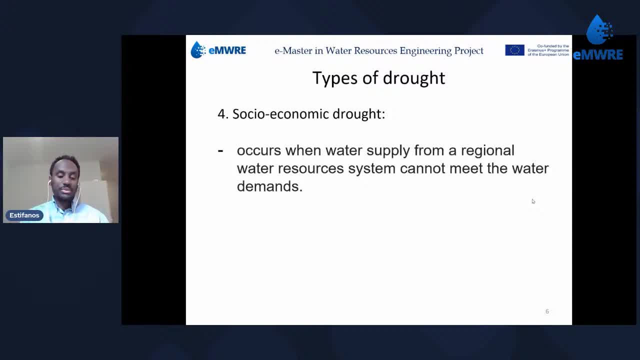 then there will be an issue of socioeconomic, For instance. let me explain using this simple plot that you see, on the bottom The y-axis is stored water in millions of liters. This is for the city of Cape Town. This was a really huge issue. 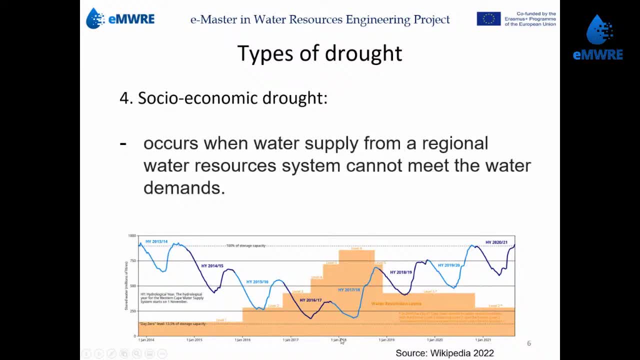 For instance, in the middle of 2017 and until 2018,, you see that the stored water has reduced substantially And the city was struck by severe drought event And officials were forced to reduce water usage even by more than 50%. 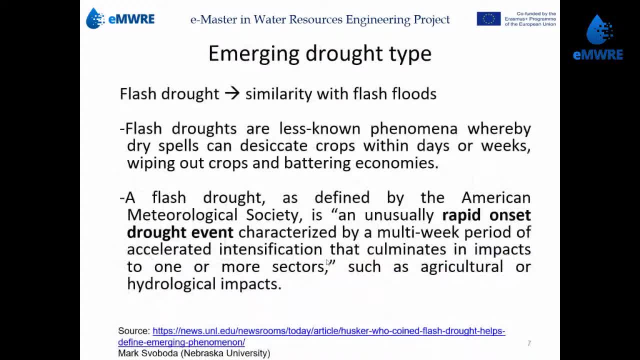 So this is what we call socioeconomic drought, And there are also some emerging drought types, which we call them flash droughts. This is similar with flash floods because they are quick ones, And this phenomena is less known. It's an emerging one. 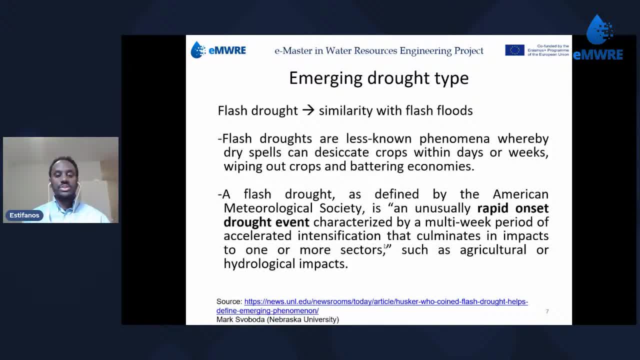 And it is defined by the American Meteorological Society As unusually rapid onset starting of drought, even characterized by multi-week period of accelerated intensification of this drought event. Therefore, usually we assess drought using monthly time staple precipitation or water balance value. 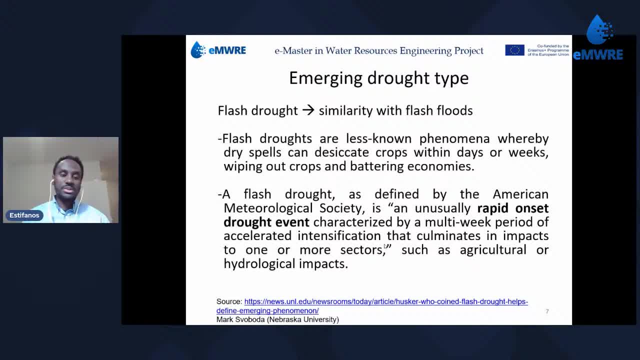 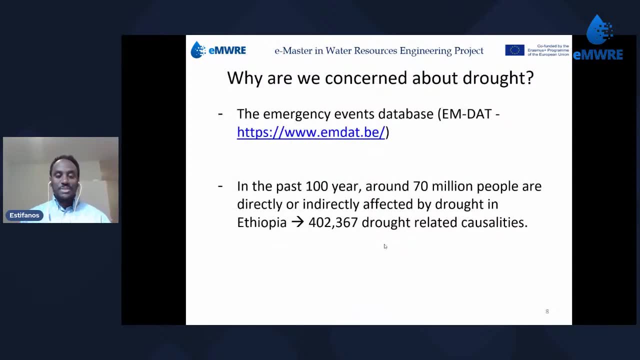 But due to these flash drought types now we are forced to go even to a lower resolution, let's say, at even weekly basis. Therefore, drought is a very complex and a very important aspect that we need to study in detail. But to give you an idea, 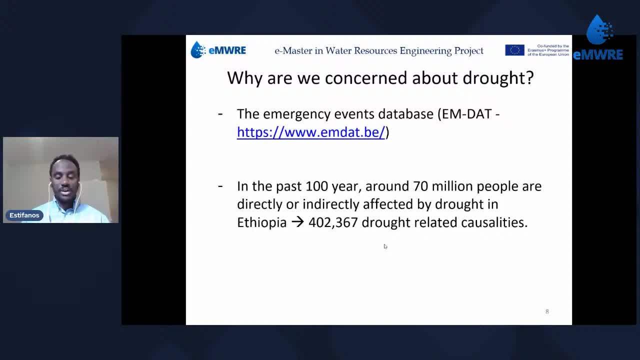 why are we too much concerned about drought? Because, according to the Emerging Events Database- you can find the link in there- In the past 100 years, for instance, 70 million people are directly or indirectly affected by drought in Ethiopia. Imagine that's a huge number. 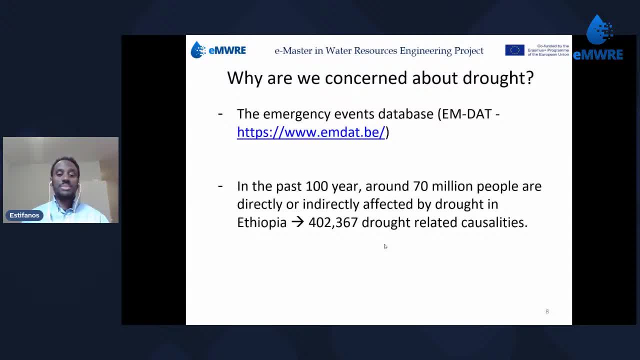 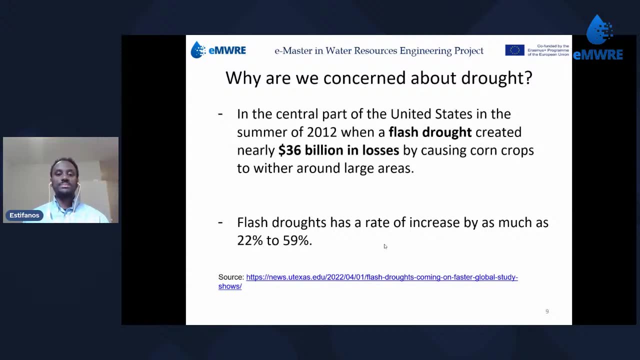 And, above that, more than 400,000 people are affected. There are drought casualties which are reported More than 400,000.. So it's a huge problem in the world, especially given the effect of climate change, making drought more intense and frequent. 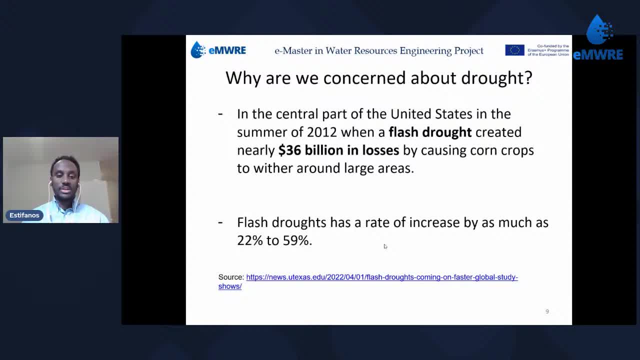 And according to also the United States data, in 2012, a flash drought caused nearly $36 billion of loss because this flash drought made the corn crops in a huge agricultural area to wilt and desiccate. And according to even recent study, 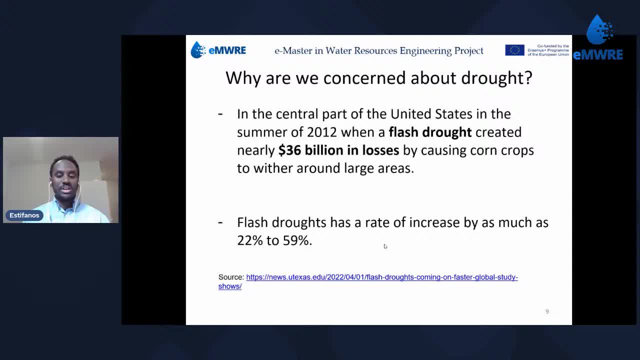 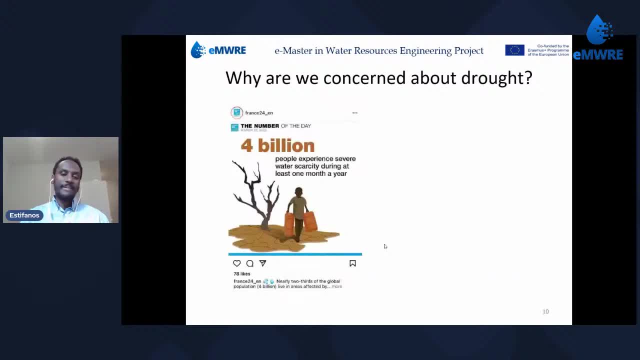 these droughts are becoming more frequent and their rate is increasing by up to 22 and 59%. That's a huge number And also media coverage is giving it more attention. As you can see, France 24, The Guardian is more giving attention to drought. 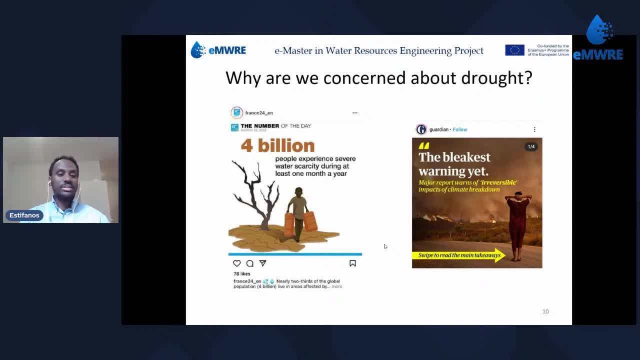 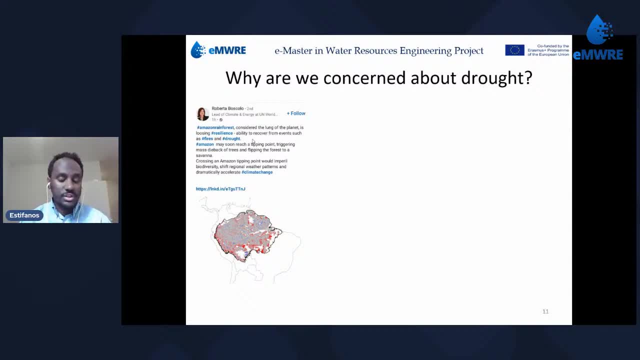 because it's becoming the dominant feature in this world And one of the leading researchers, Roberta Boscolo, also a lead climate energy scientist in the UN. she also discussed about this. the Amazonian rainforest- the biggest rainforest. it's losing its resilience due to huge wildfires and drought. 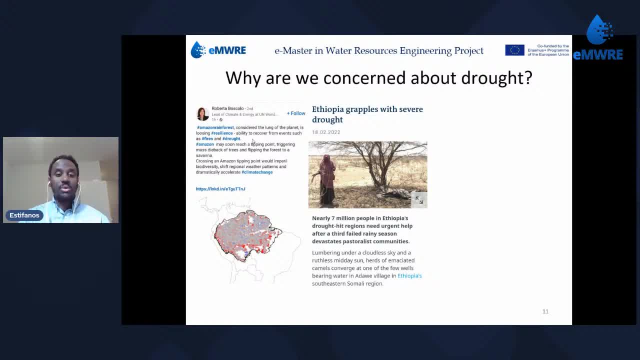 And recently, even two months ago, still it's ongoing on. nearly 7 million people in Ethiopia are affected by severe drought and in need And there are also some illustrations by some artists that if this continues, unless we mitigate it and find solution for it. 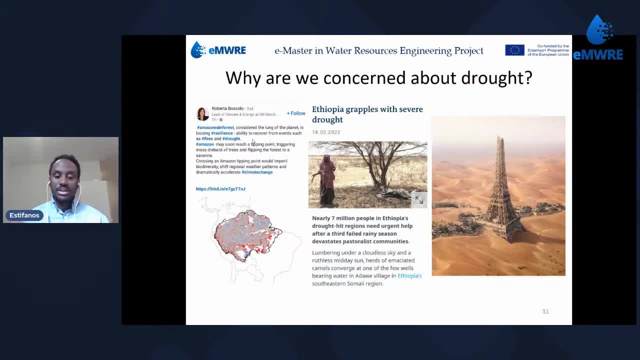 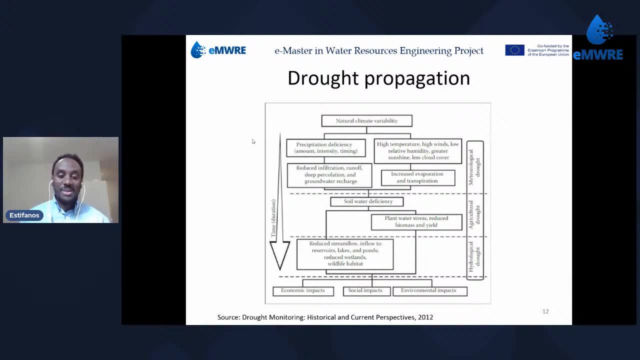 then even cities, such as the beautiful city of Paris. it can even become a desert area, given the impact of climate change increasing and drought prevailing in the future. So I don't know what will motivate you more than this. I'm motivated, And that's why I have decided to study drought in great detail. 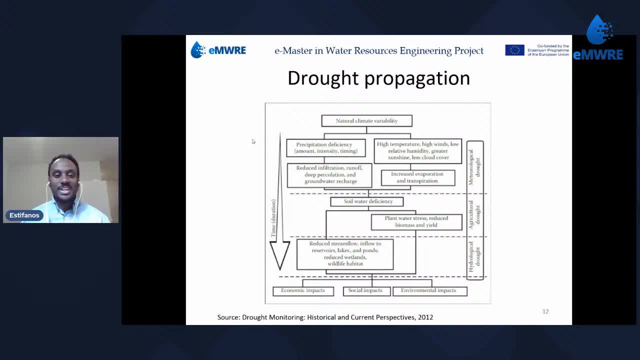 And all my research is drought, as Amani explained to you. And now we discussed about the different drought aspects, the different drought types. Now let's go for the drought propagation. So first it starts with deficiency in precipitation, So the amount increases. 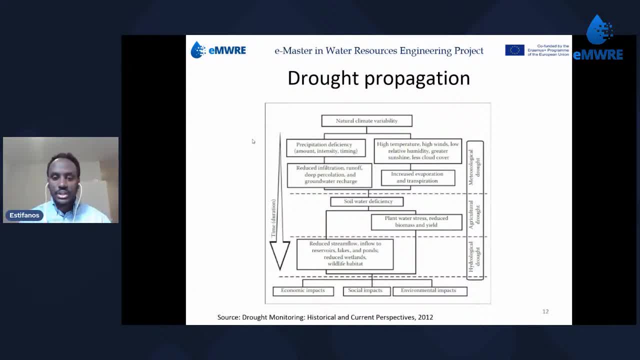 evaporation increases, that leads to meteorological drought that you see here And then if there is no water precipitating and evaporation is increasing, then there will not be any soil water. The root zones will not have sufficient water for the crops to survive. 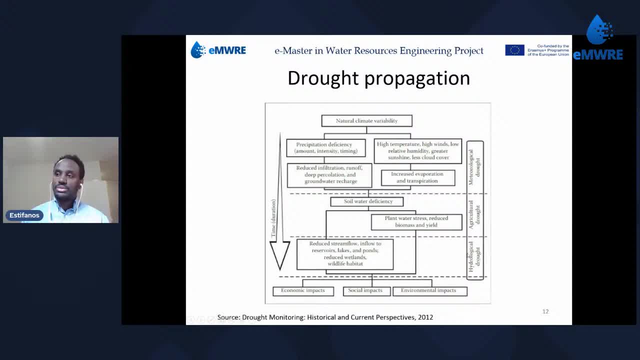 This leads to agricultural drought And finally, this will also lead to where, if there is no water infiltrating to the groundwater system, or water leading towards the streams, then this will also lead to what we call hydrological drought. And then, finally, if all this happens, 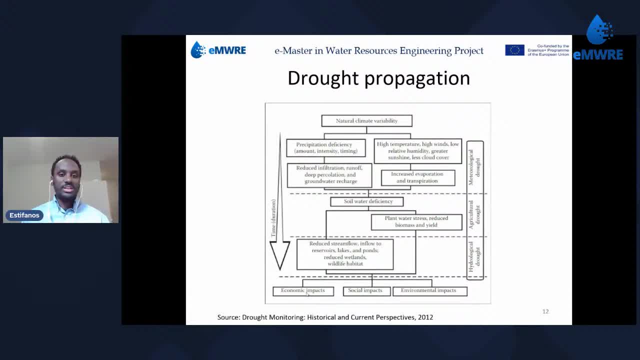 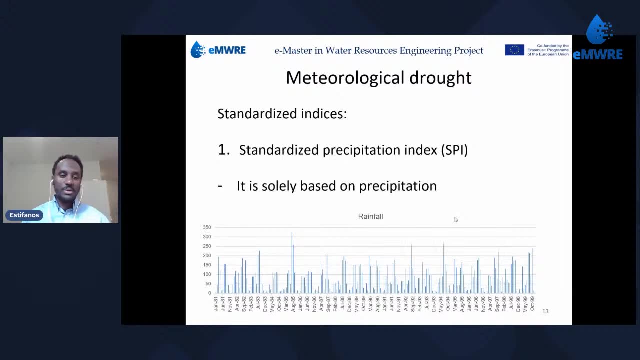 then, of course, people will not get sufficient amount of water in their taps. So that's what we call the socio-economic impact of drought. Okay, So today's main topic, that is about indicators. How do we assess this- meteorological and hydrological droughts- using drought indexes? 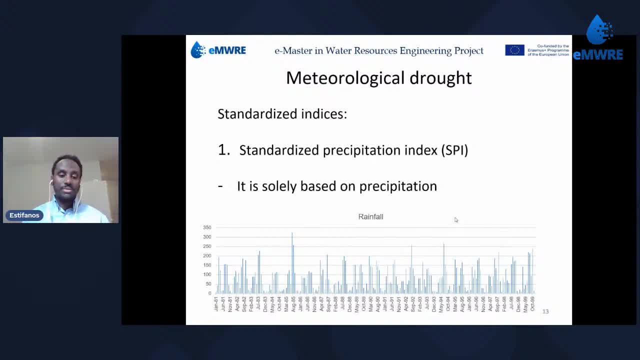 There are different drought indexes, but today I will focus on the standardized indices because they are widely used ones. So to begin with, I will start with standardized precipitation index, the well-known one, SFPI. It is based on only precipitation, So if you have a precipitation data and then using that, 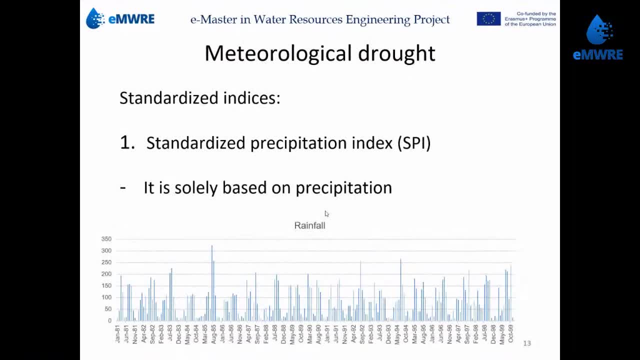 you can assess if a given year, at the given location, there is a drought or not. If you take a look into this rainfall data, for instance- this is a data from Ethiopia, for instance- there is seasonal variation, but in some cases it becomes really low. 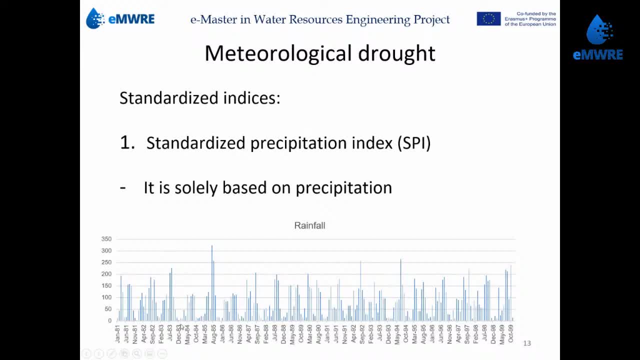 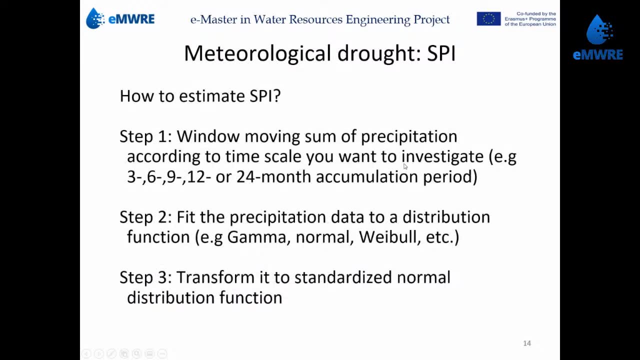 Of course there is a seasonal variation, but it becomes really low. Is that low a drought period or not? We can assess it Using this drought index. But how do we estimate it? So using drought index, SFPI, But what is the basics or the theory behind it? 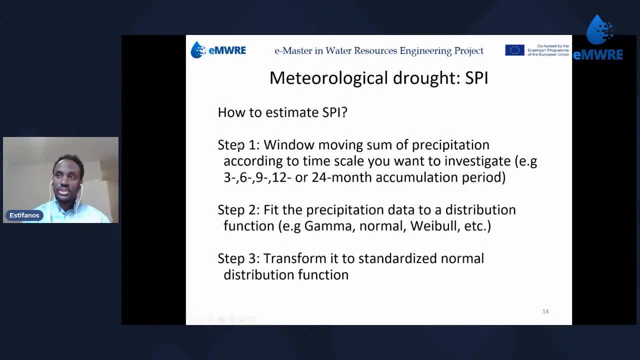 It's very simple. Let me explain it to you using just three steps. First, you have a precipitation data And then, after having that data, you perform moving window some of the precipitation. Let's say, if you want to assess at three. 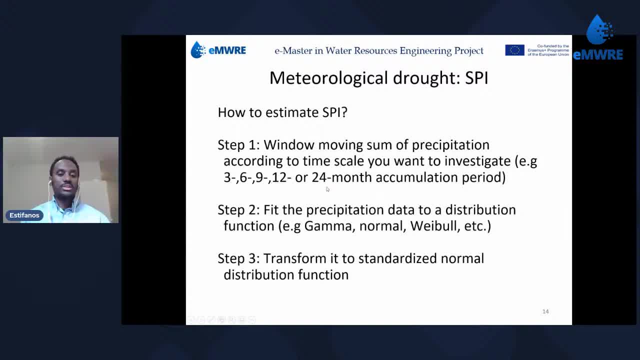 a quarterly basis or at a yearly basis or a two year basis. then you sum the precipitation in a moving window. Okay, After having that, you fit it to a probability distribution function. It can be gamma, It can be normal. 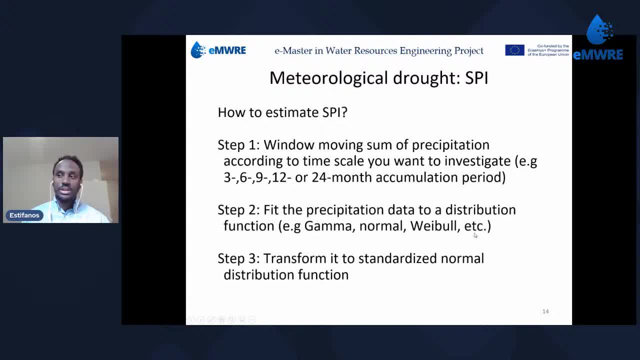 It can be Weibull distribution or any other. But how to choose this? There is also a methodology which I will show you in the next slide And then, after having this fit, then you go to the next step, where you will transform this. 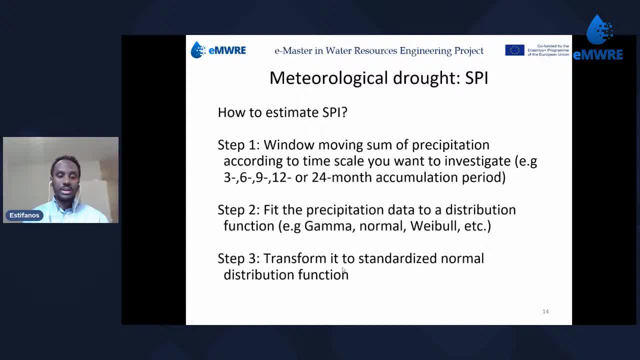 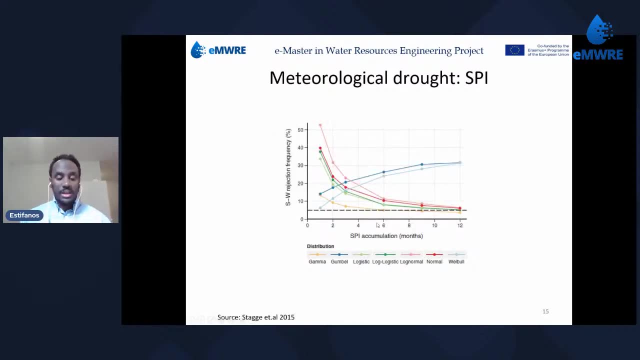 into a standardized normal distribution function, That is, it has a mean of zero and standard deviation of one. In that way you can compare these values, especially in temporally, and they are standardized ones, So to compare and select appropriate probability distribution function. 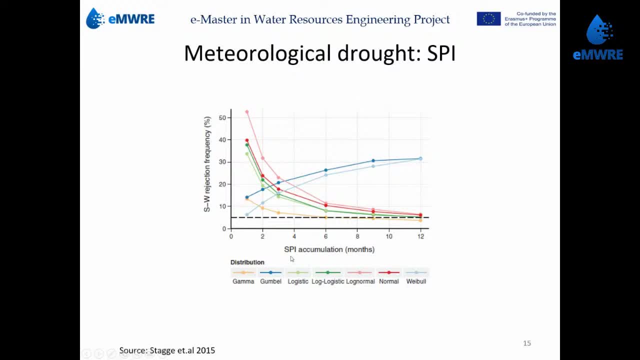 for instance, according to Studge 2015,. he compared for the whole of Europe. He made a research for the whole of Europe for different accumulation periods. He tested the Shapiro-Wilk rejection, The Sharpe-Wilk rejection frequency. Okay, 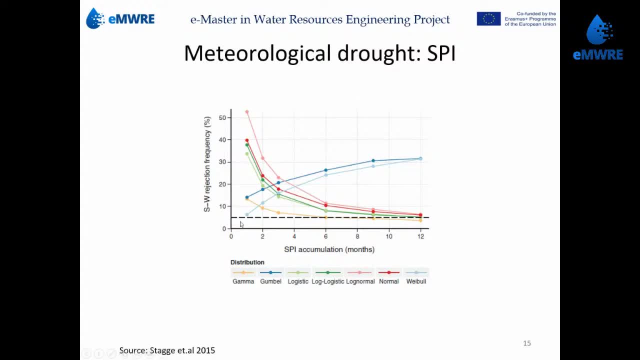 Shapiro-Wilk, It's a, it's a goodness of fit test And if a precipitation, the accumulated precipitation can be well represented by any of these distributions. So the lower the rejection, the more the appropriate distributions, As you can see. 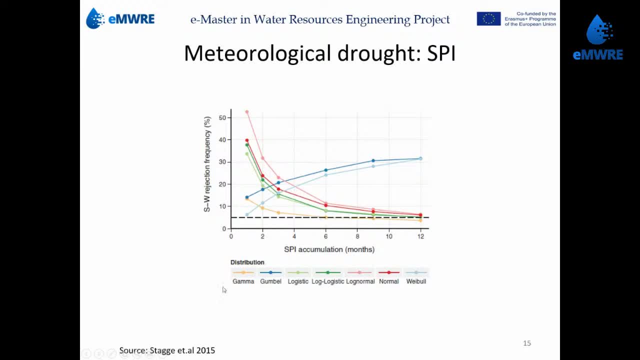 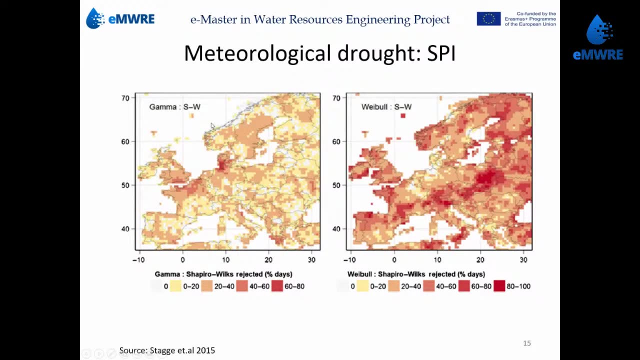 the gamma has a lower rejection frequency. due to that, we usually use gamma distribution, And this makes a significant difference. by the way, For instance, if you use gamma distribution and if you use Weibull distribution. look at the difference. 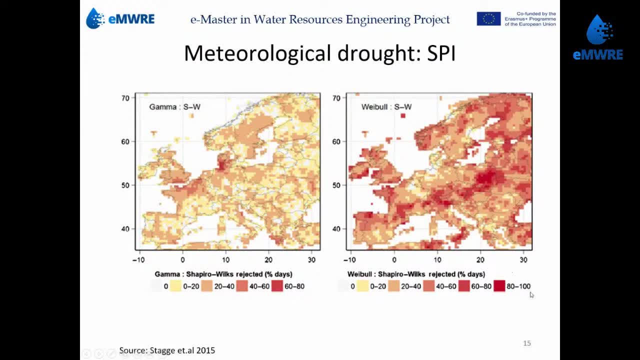 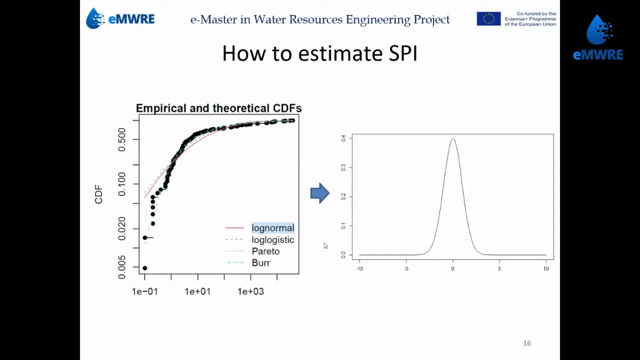 the rejection frequency. Now it's even up to 80 to 100% for Weibull, but for gamma it's very low. Therefore, due to that, selecting appropriate distribution is also very important. So, to summarize all this, when you calculate this standardized indexes, 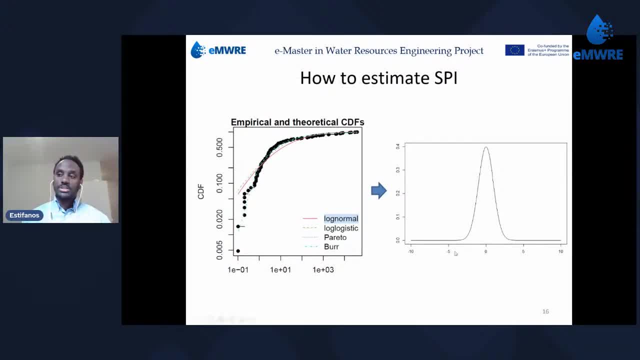 okay, any of them. that I will explain later as well. The concept is very simple. You feed the, the accumulated precipitation or let's say, water balance value that you have, to a priority distribution function and then you transform it into a standardized normal distribution function. 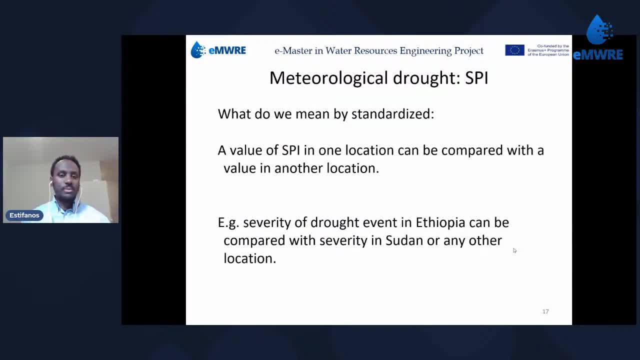 But the question here is: what do we mean by standardized? It has a very important meaning, That is, a value of SCPI in one location can be compared with a value in another location, even at any time window. Okay, For instance, 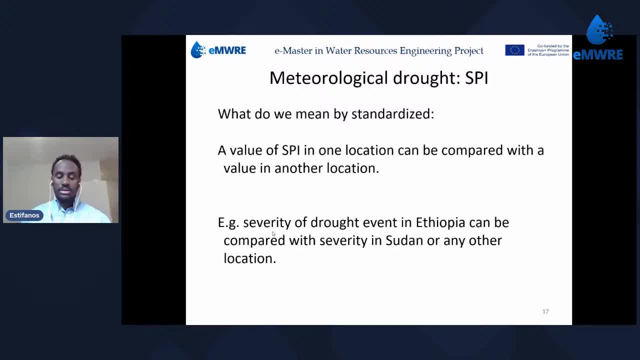 a draw: severity of SCPI value of minus two here in Belgium and a severity of, let's say, in Sudan. let's say, if it's minus one, then the one in Belgium is more severe than in Sudan. So you can compare them, because both of them 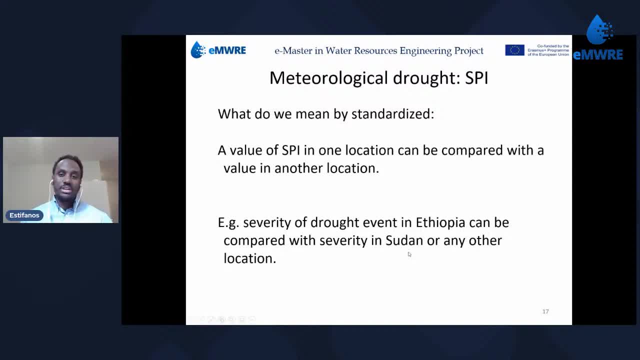 they are based on one approach. Therefore, a standardized indexes are gaining more attention due to this nature. Now, let me give you some examples. Okay, Just the one example that I have, By the way, this is a. this is: 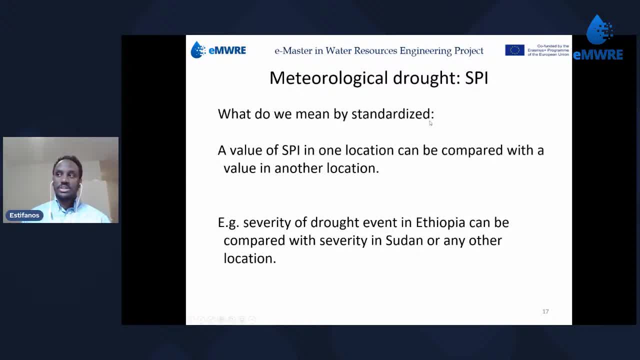 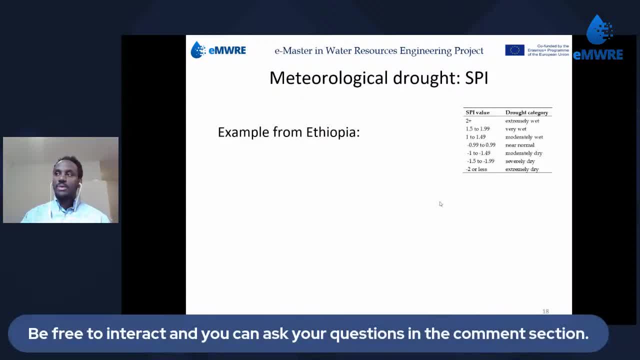 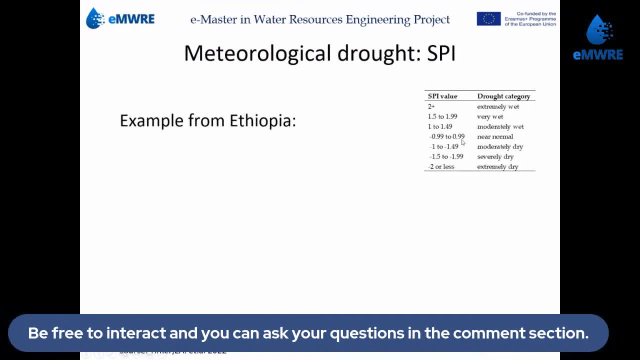 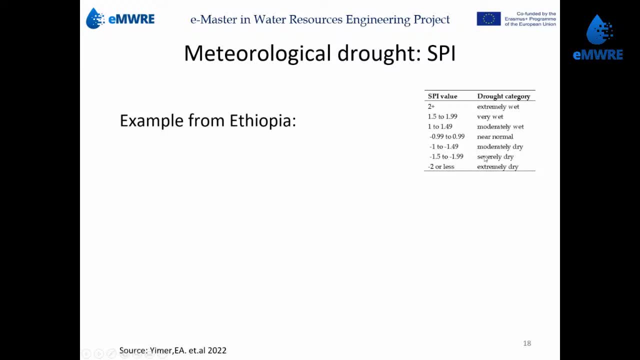 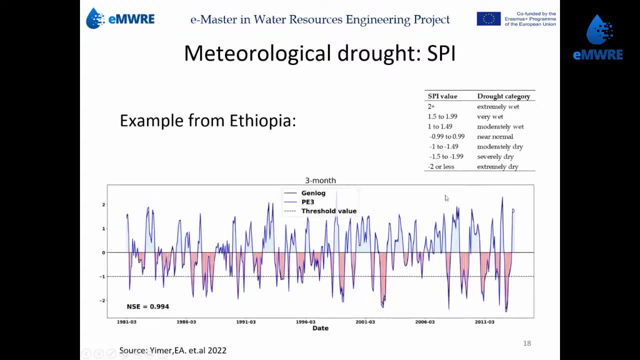 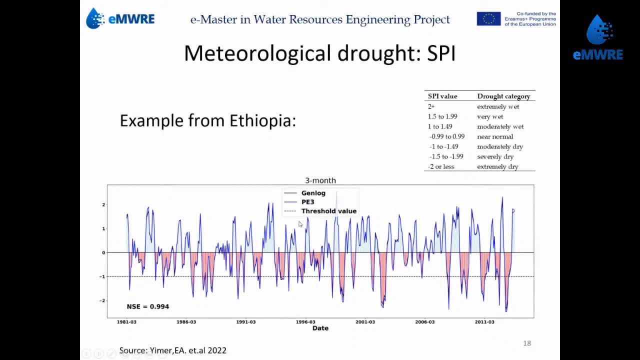 out of my paper that i have published recently that you see at the bottom. but forget about the comparison that i made between the distributions, but look into the shaded areas. the red ones stands for drought parrots and the blue ones stands for wet with parrots. okay, as you can see, there are a 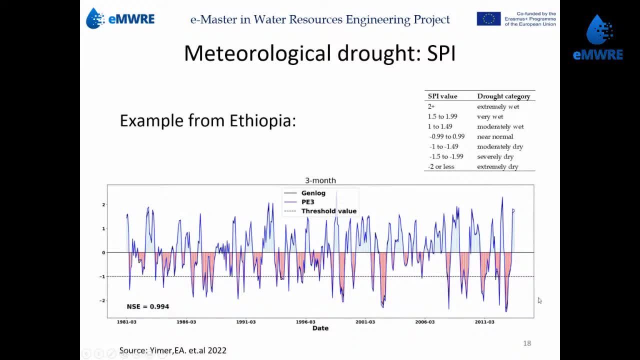 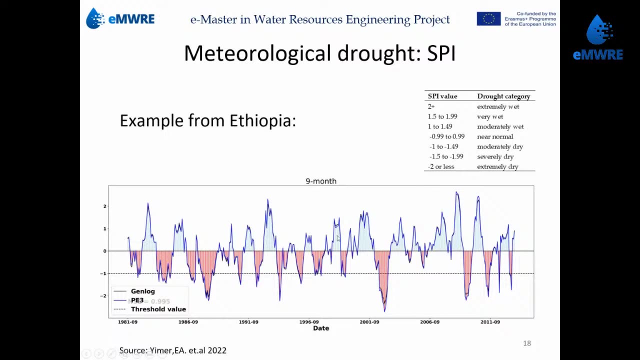 number of drop packs, especially in here. it can even reach up, be beyond minus two. so it's becoming more extreme, dryer, extreme um drought event is happening. this is for one aggregation level, let's say three months. it can go up to nine months, for instance, when it go, when you go to higher. 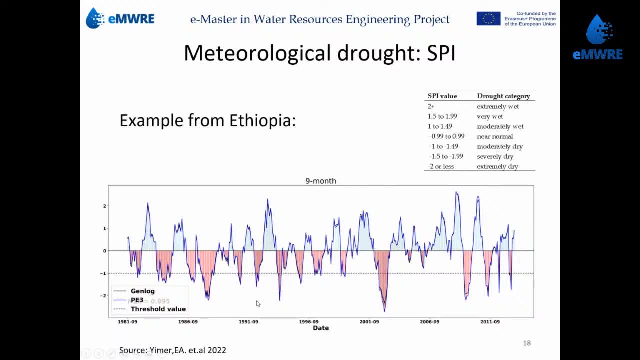 creation level: the the frequency decreases, huh. as you can see, if i take you back, there are a number of them, but when you look into the nine months there are only few. but their duration is a standard huh. so in that way you can access the different drop types using these drought indexes. 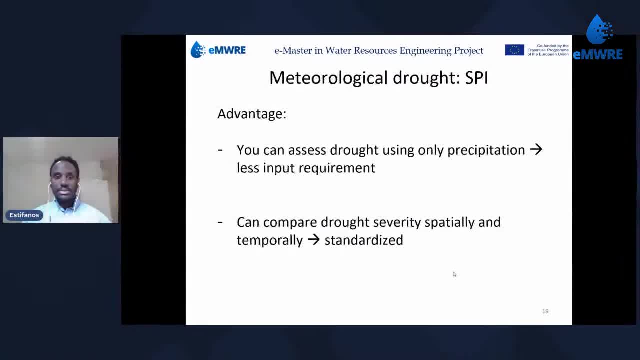 so now let's discuss about the advantage and disadvantage of the different indexes. okay, for instance, for a standardized precipitation index, it's only based on precipitation, so you only need to provide the precipitation data and then you can access drought using that. that's one input, only one input. the other drought indexes. they might need more inputs. 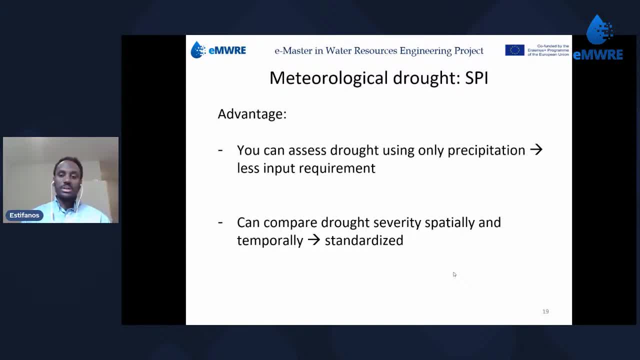 for example, a about trade für radiation, relatively humidity, wind speed, uh, machimum temperature, minimum temperature and so on, but in here you only need precipitation. so that's one advantage and also it's a standardized one. you can compare it spatially and temporally. that's another. 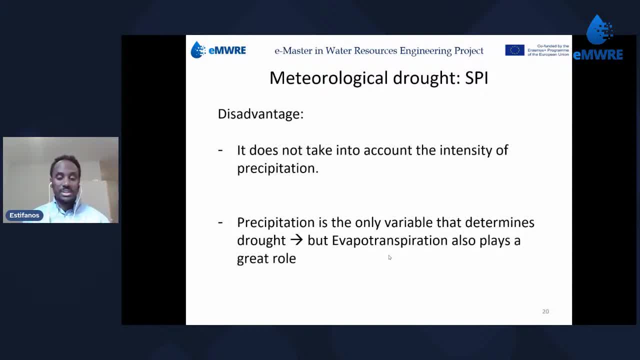 advantage, but it has also disadvantage. it doesn't take into account, for instance, the intensity of precipitation. it just take into account the total amount of precipitation. for instance, is it hundred taking place in an hour, or is it in two hours or in a day? that will make a difference, because the 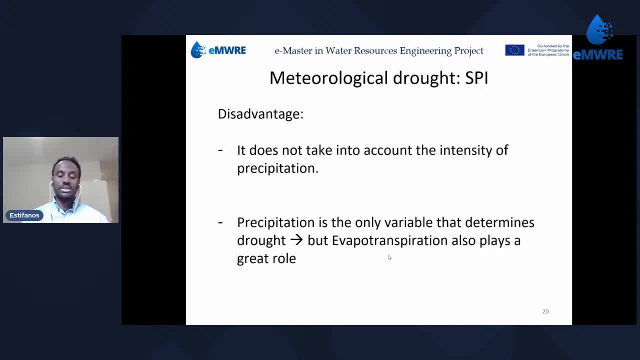 amount of water reaching the rivers is different for the different intensity groups. also, there is this precipitation index is based on only precipitation. it doesn't take into account other variables, for instance evapotranspiration. this is an issue because evapotranspiration can be really significant and determining for drought in most part of the world, especially, for instance. 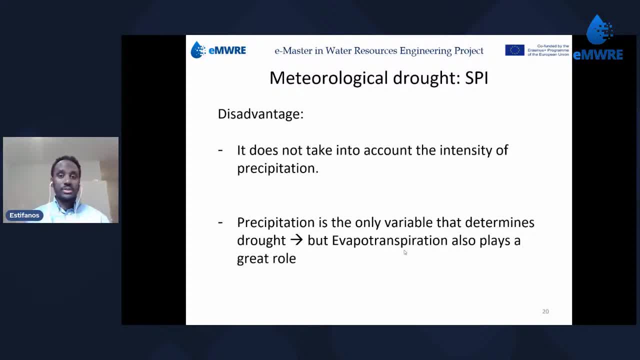 in in dry areas where evapotranspiration is really high, for instance at 1000 millimeter of precipitation, and then if 600 millimeter of them is corresponds to evapotranspiration, then if we just assess using precipitation, that doesn't make full sense. you have to take into account also other 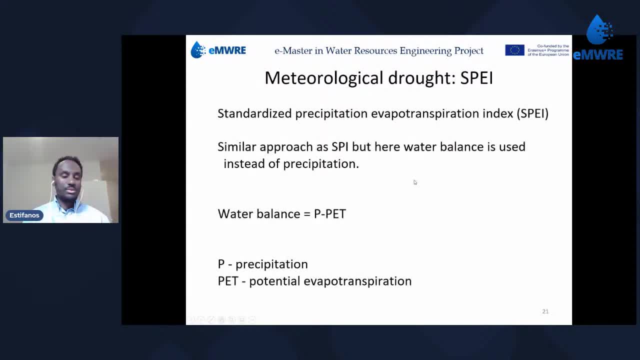 variables. That's why researchers Vincenzo Serrano and his colleagues came up with the idea of standardized precipitation evapotranspiration index that you see in here. it does similar approach as a CPI, but here we don't use only precipitation, but we use water balance. that is the difference between. 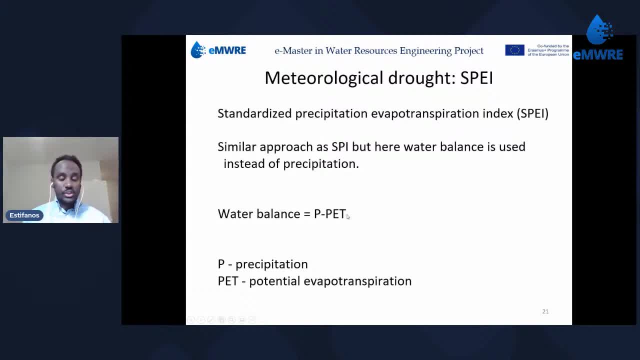 precipitation and potential evapotranspiration. so potential evapotranspiration, you can, you can calculate it using Pen Marmontes or you can calculate it using healing heart, gr, trading ormeter of toronto, het or tiller method. there are a number of them. 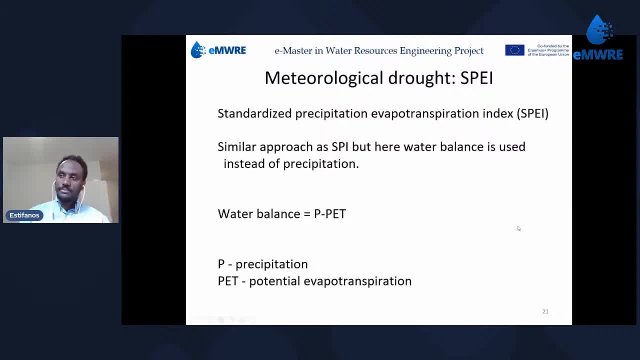 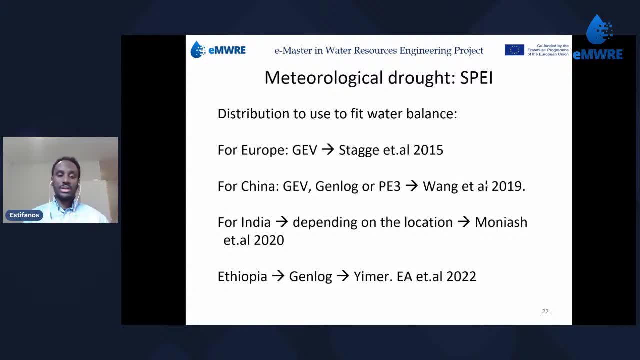 according to the data that you have, you can calculate that and, as I explained for CPI, I showed you that gamma distribution is appropriate one, at least for Europe and for most parts of the wallet, but for a CPI there is no conclusive notion. for instance, for Europe, the studies suggested 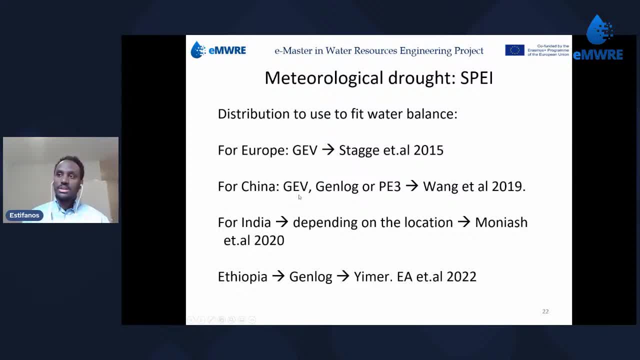 general extreme value distribution. for China they said it can be GEV, generalized logistic or Pearson Type 3, and in India they said it depends on the location. In some locations it's Pearson Type 3, in the others it's generalized logistic And recently 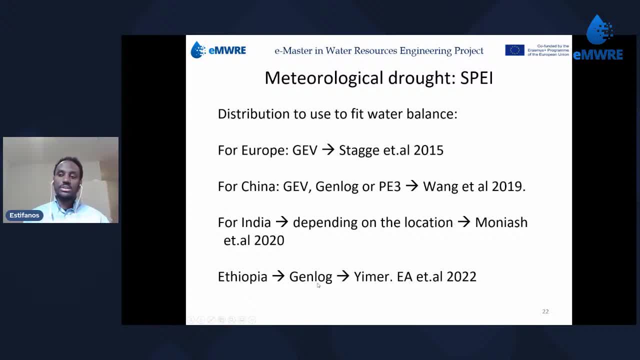 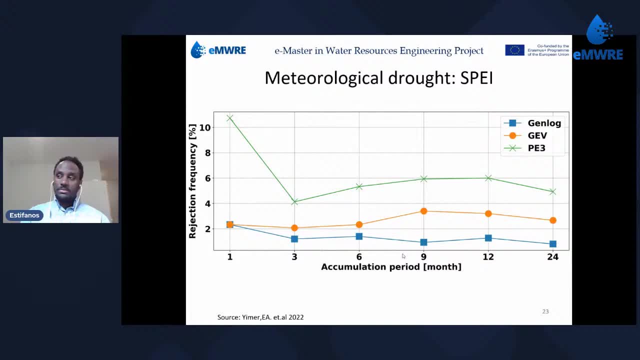 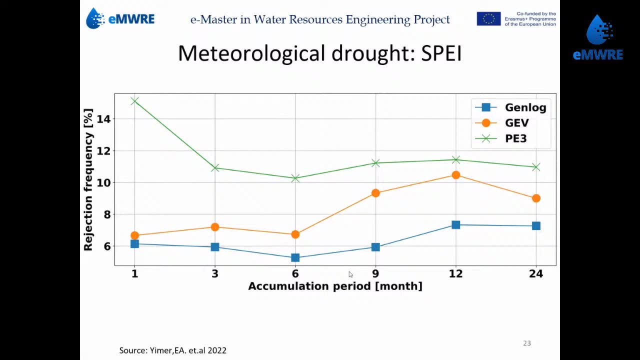 I did research with my colleagues and we found that generalized logistic distribution is appropriate to be used for Ethiopia. Okay, now, this is based on. this is from my paper, so I compared different methods. Okay, Goodness of feed. test Shapiro, Wittes test Andersen-Darling. 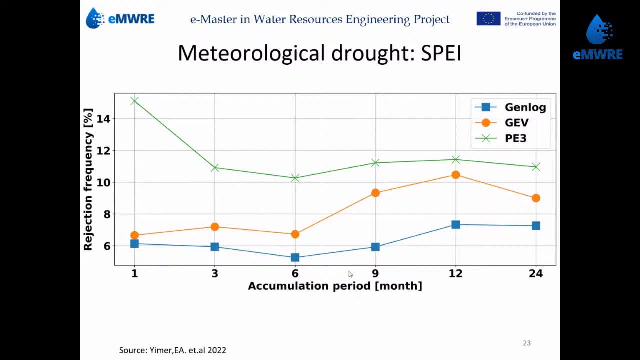 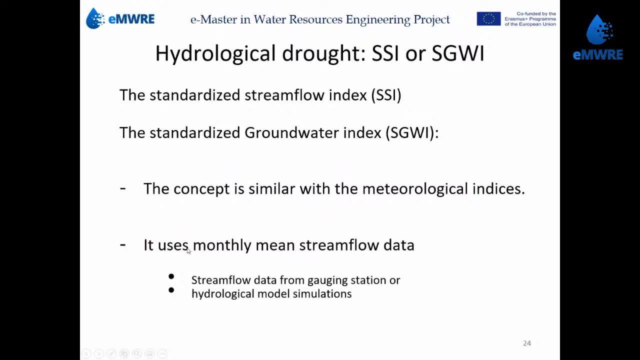 and Kolmogorov-Smirnov goodness of feed test and we found that generalized logistic distribution has the lowest rejection. that's why we chose it. Okay now. we discussed about meteorological drought indexes. now let's discuss about hydrological drought indexes- The same. 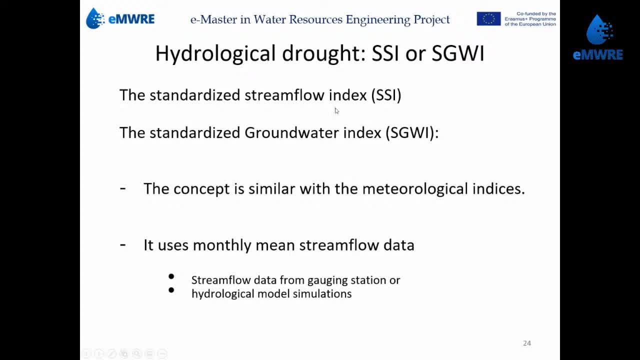 approach is used in this: standardized indexes. but the difference is the input. If you want to to access, drop in, let's say reverse. you use monthly mean streamflow data, for instance, and then you follow the same procedure: you fail it to provide a distribution function and then you transform it to a standardized normal distribution function. the same applies. 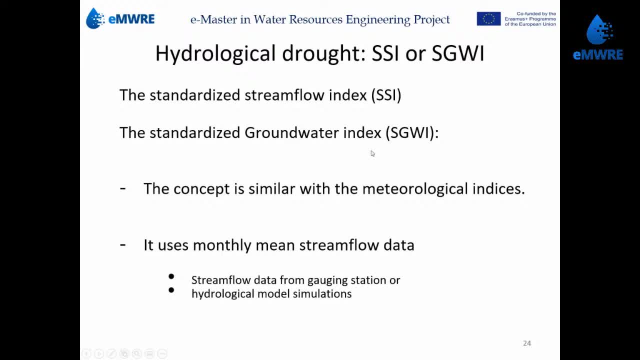 for groundwater. if you have groundwater head data, hydraulic head data or fluxes, you can access using the same concept. okay, for instance, let's go for streamflow, uh, standardized streamflow index. for that you need to streamflow data. one you can get it from gating station, the other you can. 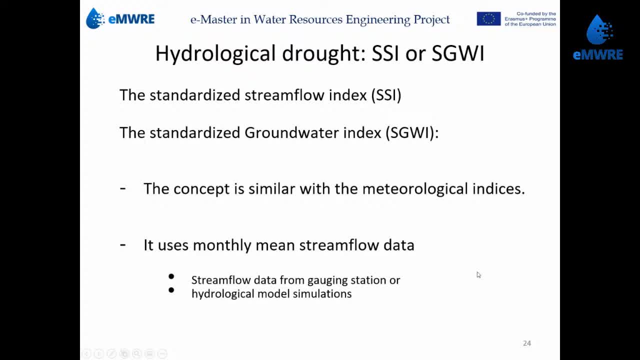 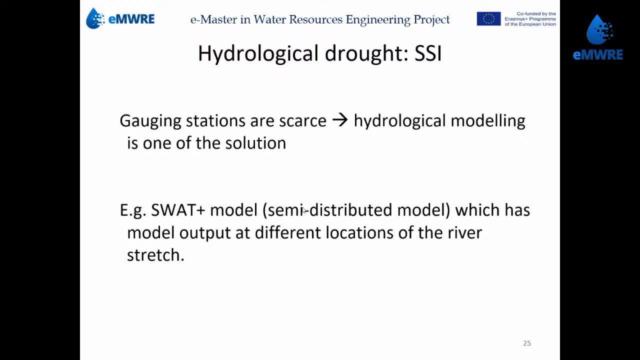 also perform hydrological model simulations. why? because gating stations are very scarce. that's why we prefer to go for hydrological modeling. that can be one solution. for instance, we use the soil water assessment tool, which is a semi-distributed model, which has a model output for different river stretch in a given catchment. okay, so first you can. 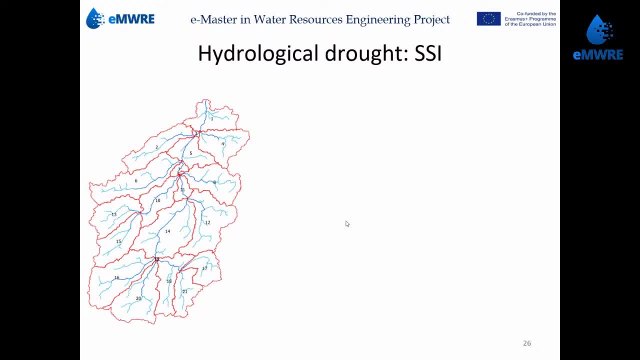 calibrate the model. if i have this catchment- this is a catchment that i'm working on recently and uh, it's uh, in the middle of belgium- a dial catchment- if i have a streamflow data at the outlet, then if i can calibrate using this data- okay, this data i can calibrate, the i can calibrate. 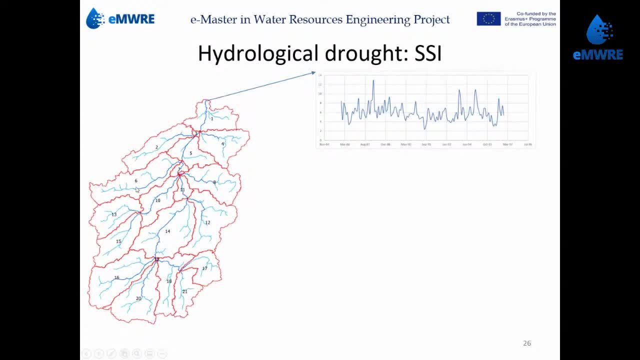 the catchment and then made it to estimate the streamflow at any reverse stretch. okay, here i can get, after calibrating and validating it, i can get streamflow data here. i can get it here. so monthly or daily time step i can get it. so ideological models can be a way forward to get more streamflow. 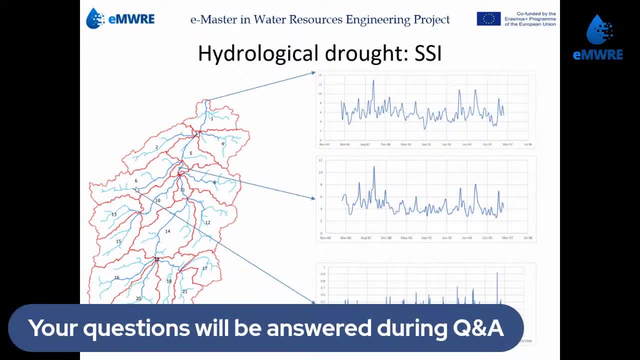 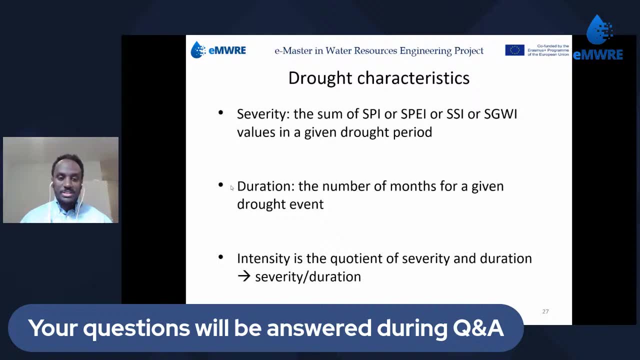 data- okay, if you don't have more gating stations- and then perform the same, the same uh approach as the other indexes, and i would like to uh end this with drought characteristics. okay, there are three main drug characteristics that you have to consider. the first one is the severity. yeah, it's the sum of the drought index that you are. 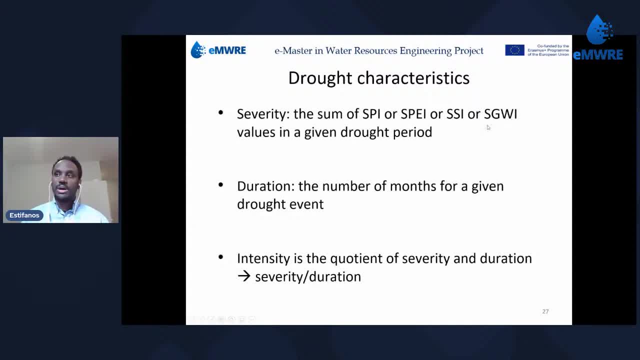 assessing it can be spi, spi, ssi or sgwi for a given period of time. for instance, if a drought happens, let's say from september 2021 until, let's say, december 2021. so from in that period, if it's under drought, and based on the growth category that i have shown you, and then you sum the spi. 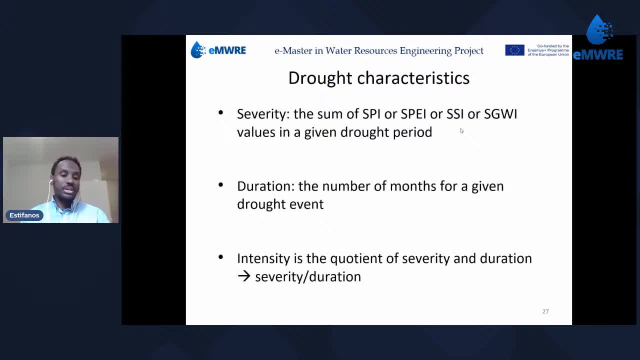 values in that period. okay, at monthly time. step you sum them. that will give you the severity, how severe it is, okay. and then the duration is from the starting until the ending period. what is the? the time lapse between the starting and the ending of the drought event and the 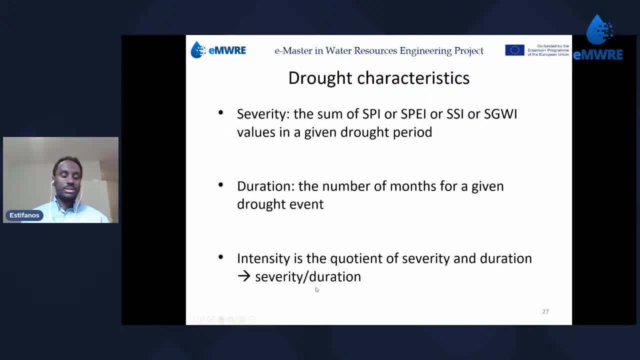 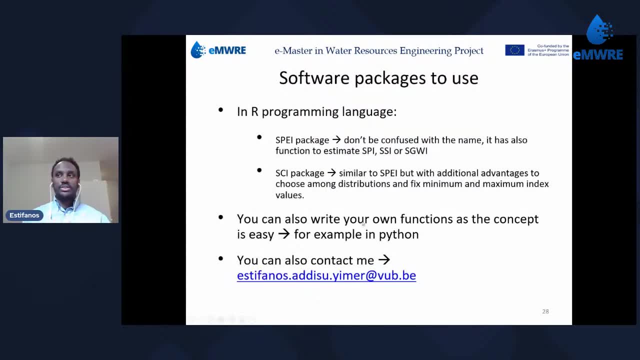 intensity is the quotient of the severity and duration, and then this will show you how severe the drought is compared to the duration and software package to use. if you are acquainted with our programming language, which is high programming, high level programming language, it's not difficult. so you can find spi package and sci package which both of them can help you to. 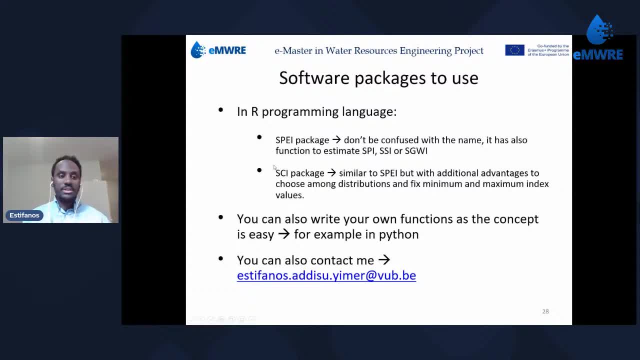 estimate these indexes very easily. okay, their idea is very easy. i have shown you so. but you can use this package- but don't be confused with the name when you see spi package. but it can also be used to estimate sapi, ssi or sgwi. the difference is that you have to give it the appropriate data. 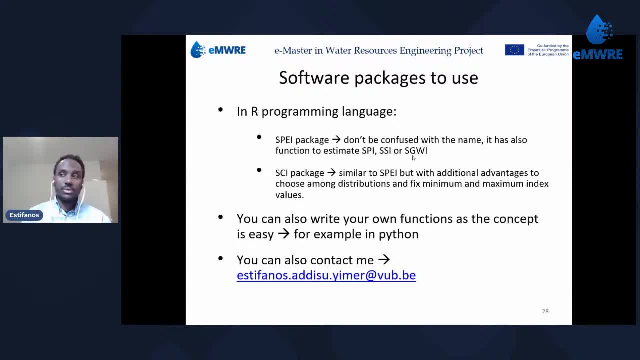 if you are assessing the standardized streamflow index, you have to give it streamflow data. if it's about a standardized groundwater index, then you have to give it groundwater head data or fluxes. and there is also a sci package. this package it has advantage because it contains different. 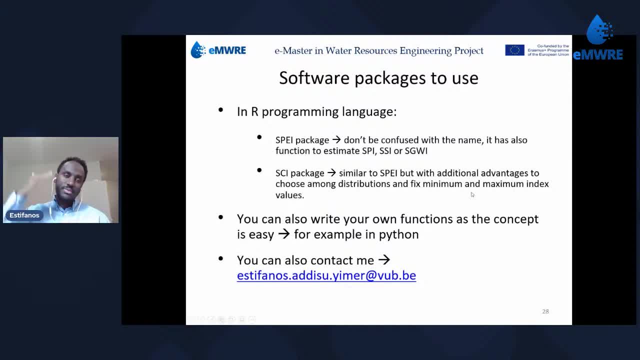 distributions. okay, you can choose different distributions. also, you can fix the minimum and the maximum- uh, drought index values. because these drought indexes, they are estimated, we feed them, so we are estimating it out of the distribution. therefore, when you go to higher values, then the probability will decrease. that it's it. you can't rely on it. it's a. there is an. 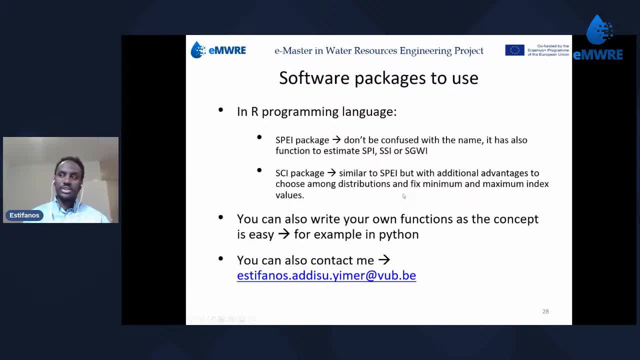 issue on the uncertainty of the values. that's why he came up stage, came up with the idea of fixing the minimum and the maximum indexes. so you can take a look at this one also, okay, in our programming language. or you can also write your own function. as the concept is easy, i have explained it to you. 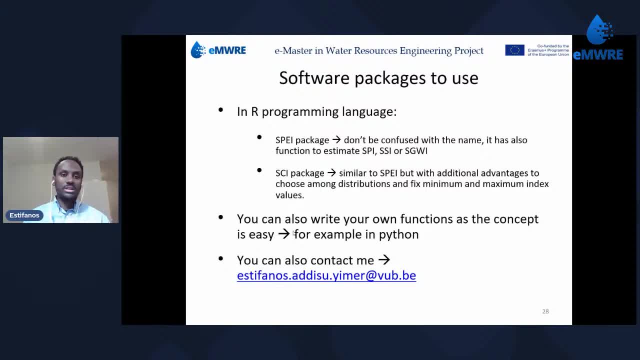 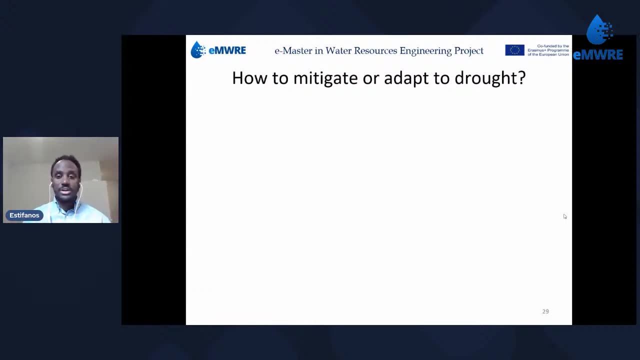 for example, in python, you can easily write this code and then function and then use it several times. or, if you want, you can also contact me. you can. you can see my email at the bottom and then i will help you further. and finally i would like to end. we discussed about drought. drought is especially given climate. 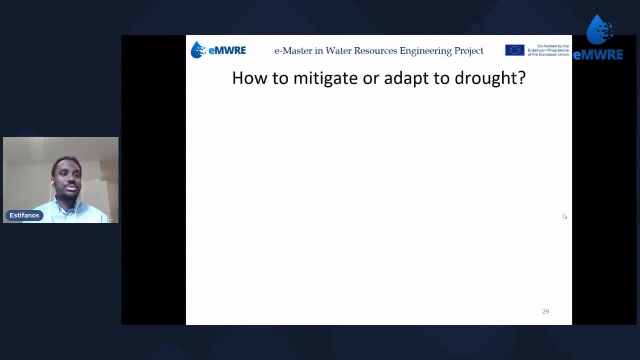 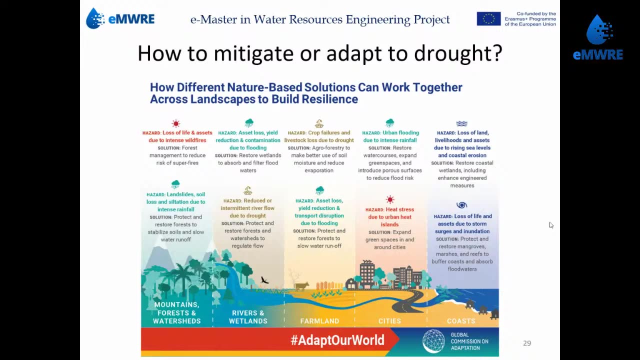 change is becoming more intense and frequent. therefore, we need to do something about it. huh, we need to mitigate it and adapt with it. and how do we do that? i would like to take you and bring you to the concept of nature-based solutions. huh, nature-based solutions are a way forward we need. 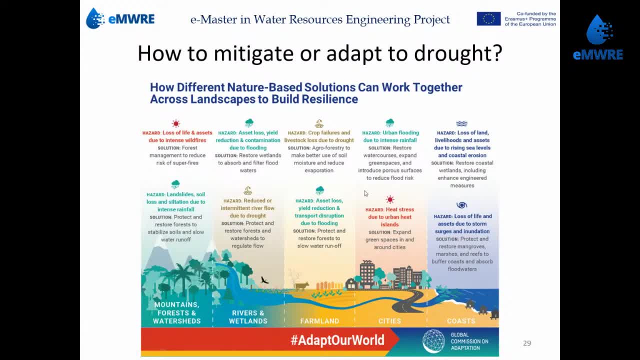 to. we don't need any more pavements here and there, but we need to find green infrastructures in the world and we need to restore wetlands so that the water can infiltrate the groundwater system, and also we need to plant uh forests. we need to have more buffer systems so that we can be resilient. 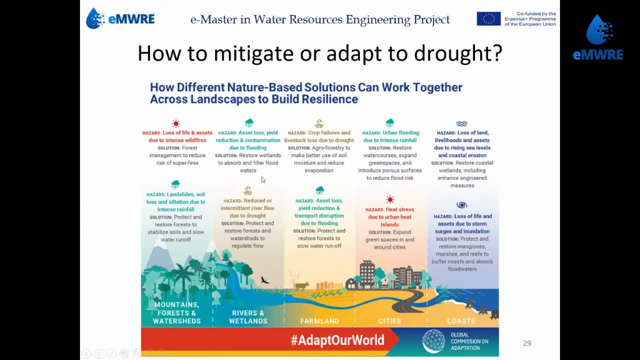 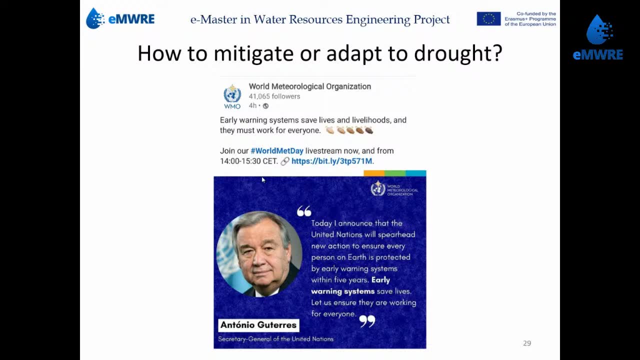 when drought is happening. therefore, that's one way, and please keep that in mind. and finally, his excellency antonio guterres, the un secretary general, also recently tweeted that early warning systems are very important because, especially in developing countries, it's very difficult to find. 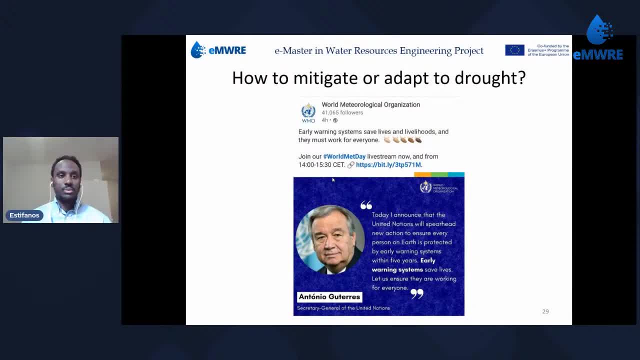 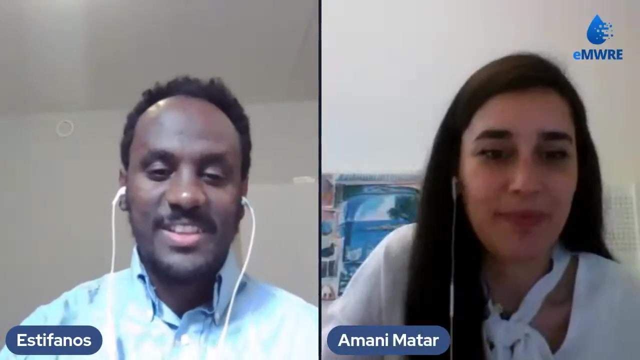 early warning systems and people who lose their crops and animals because of that. but if we can uh predict with some degree of probability and have early warning system, we can cope out with this natural climate, climatic hazards. that's all i have. thank you so much. yeah, thank you very much. uh, very interesting presentation and definitely different from the 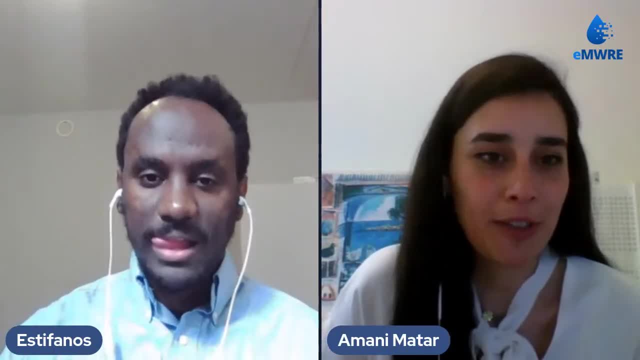 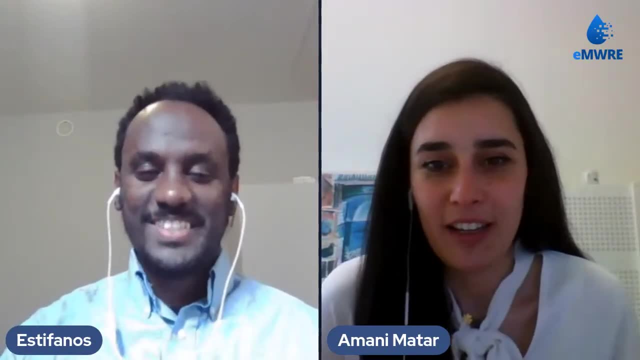 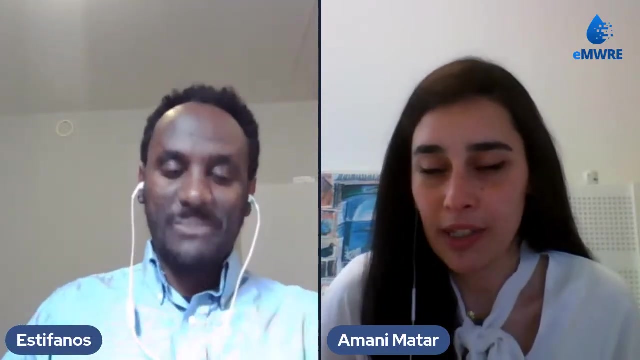 other presentations, so we were talking about floods and this time about droughts. so i think so it's very interesting to see both extremes and that we have to deal with it. um, so yes, please, if you have any questions, put them in the chat box and we can start our q a session and address some questions that we have. 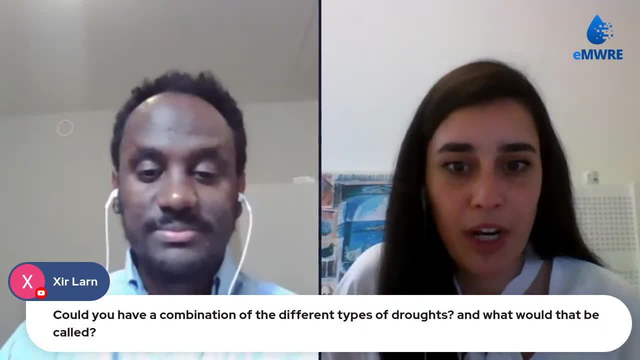 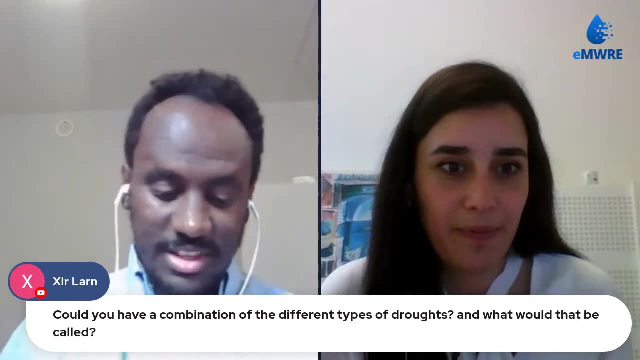 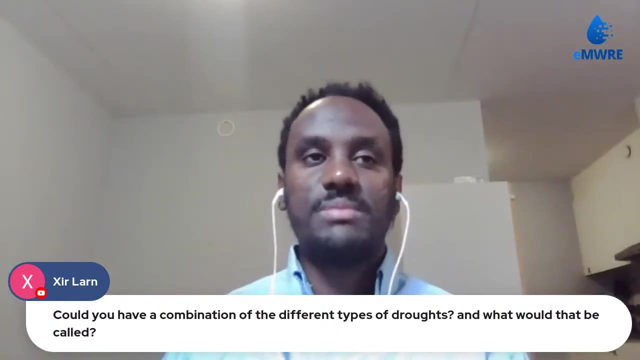 so the first question: could you have a combination of different types of droughts and what would be that called? uh, yeah, that's a, that's a good question. uh, it's uh droughts. when it happens, as i have explained, there is a propagation between them, so it starts with the meteorological and goes to 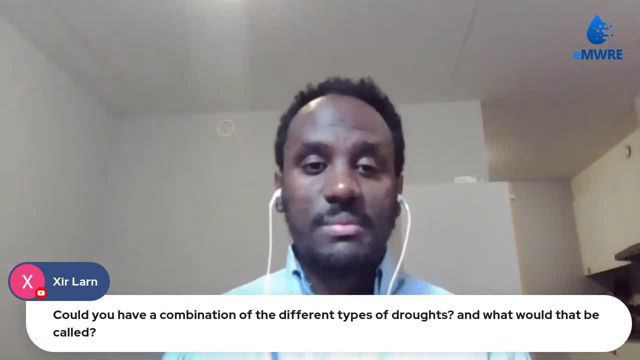 the agriculture and the hydrological. but the good thing about this: drought indexes: you can assess them using like, for instance, if you are using spi standardized precipitation index. when you use lower aggregation level- one month, three months aggregation level- you are assessing more or less the meteorological and agricultural drought. but if you go to higher aggregation, let's say 12 months- 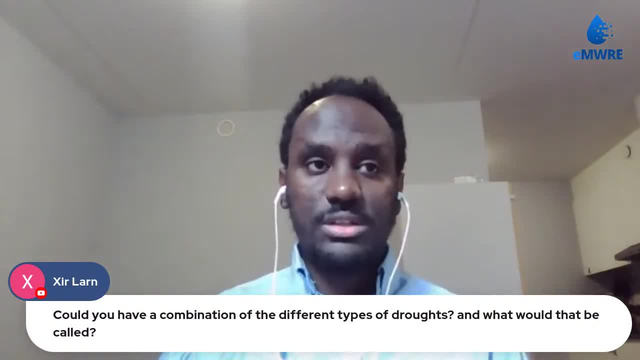 or two two yearly basis. then you are assessing more of the hydrological uh droughts. because they are, they are not uh, they don't have the mechanism to react quickly because the groundwater system, it will not be affected quickly whenever meteorological dot happens. therefore we, we can't. 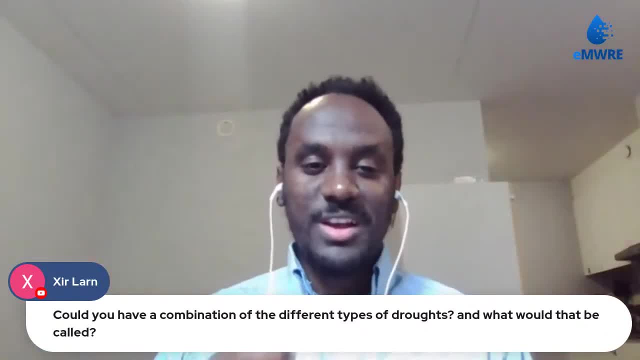 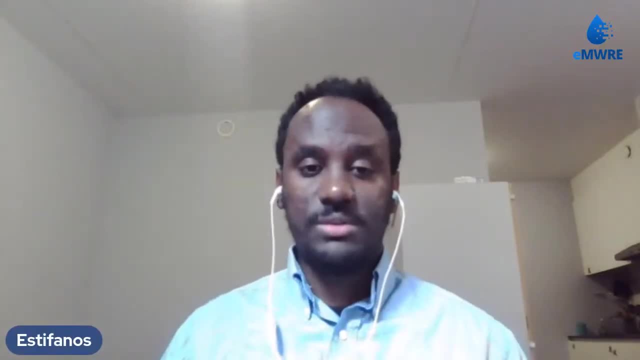 give a general name for everything, but we can assess them using different aspects. okay, using different aspects, but for sure there is a combined effect of it and that's the challenging test we have, even at the moment. that's why it's very complex. if you remember, i said it's very complex. 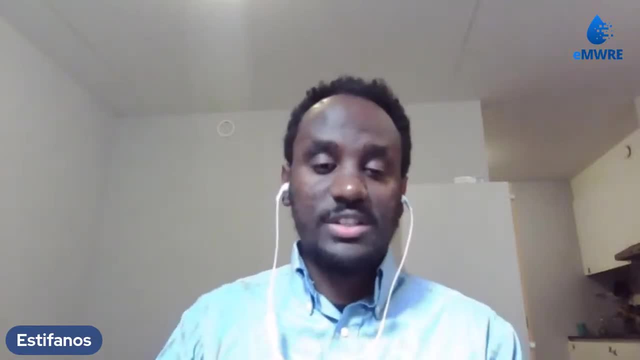 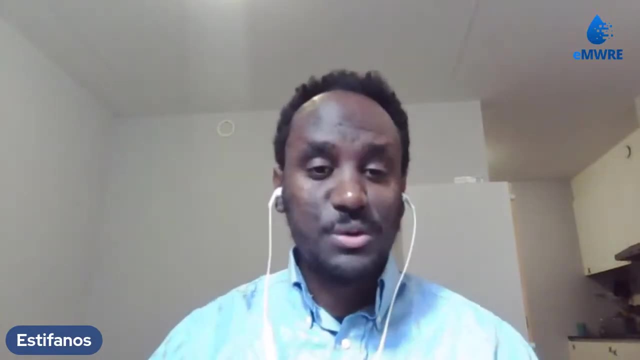 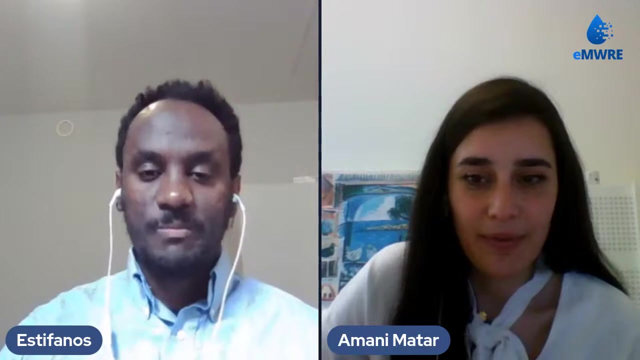 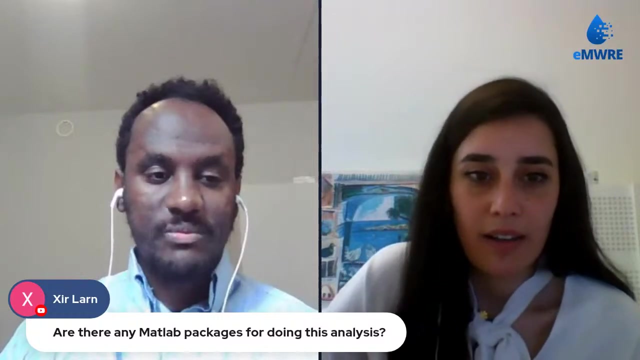 it's very uncertain, but if we can tackle the uncertainty coming from each sources, then you can. you, you can access it in great detail, but you can't give it just one name. okay, yes, thank you very much, um, i think. um. i have other questions. are there any matlab packages for doing the analysis? 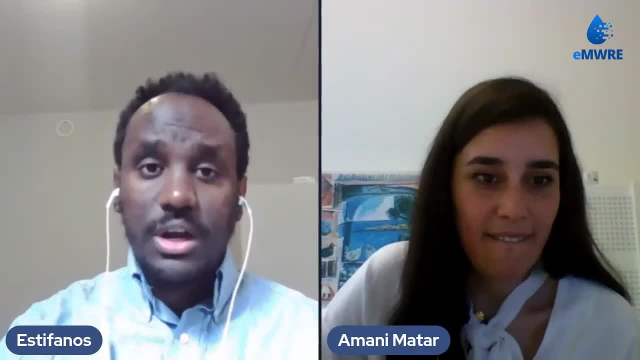 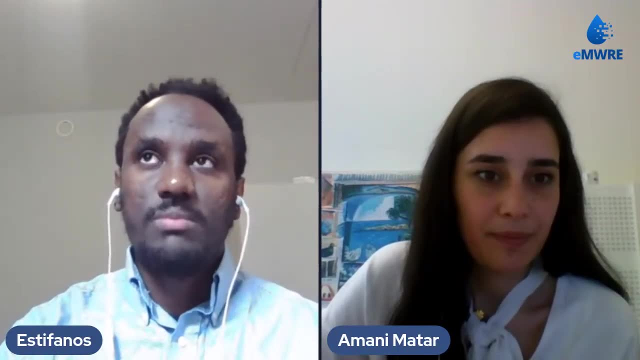 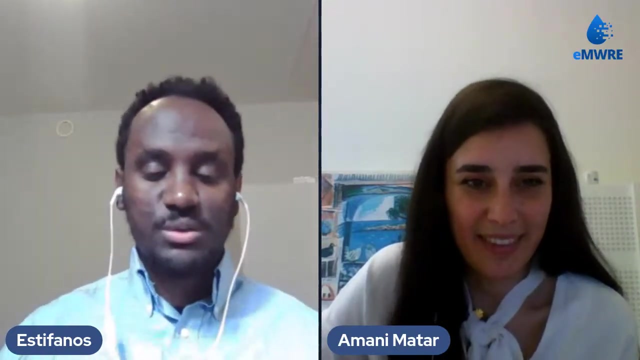 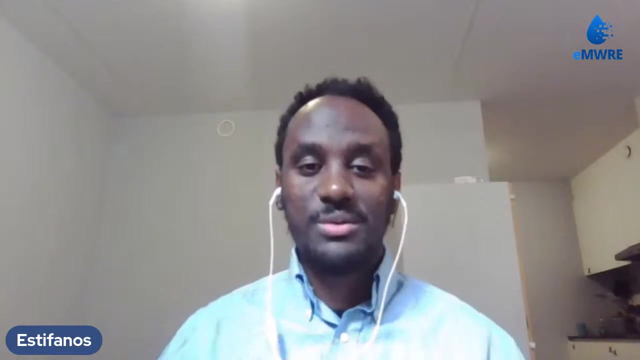 yes, there are some matlab packages so you can just especially: um, yeah, there is a guy who is developing matlab course, because matlab it's not open source and so usually for us we focus on open source so that everyone can use them. so, for instance, i developed a number of scripts using python or r. uh, so i can't for sure say the guy, but i know that there. 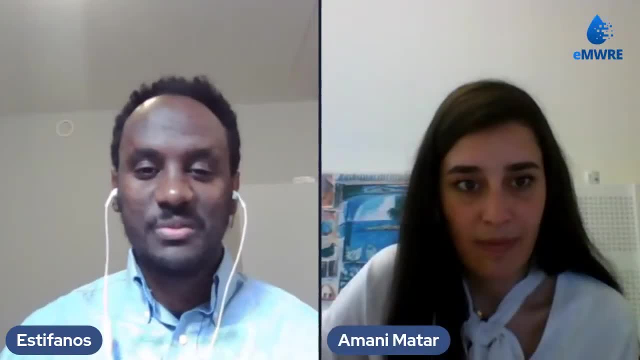 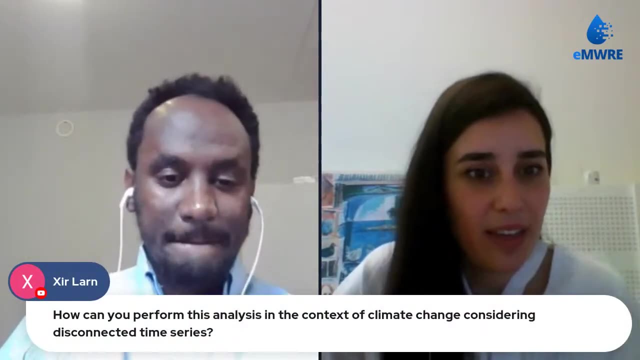 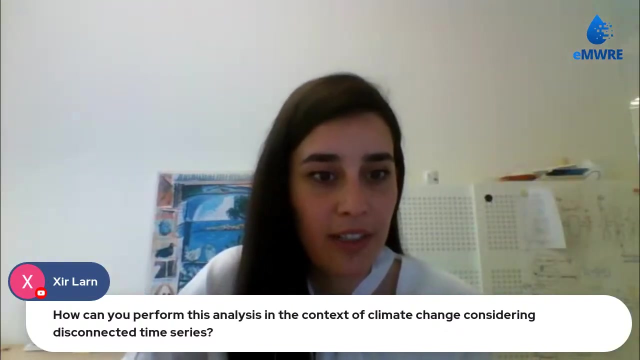 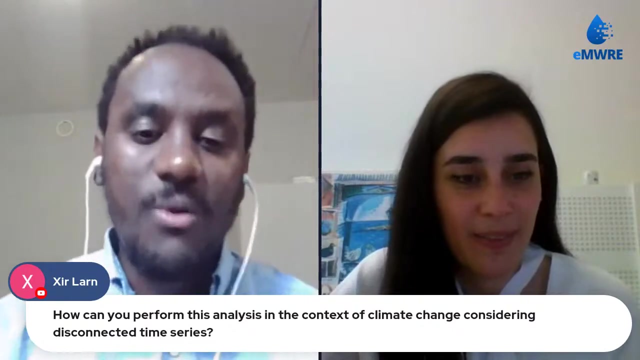 are? okay, there are. if you want, i can search and then contact me and then i can share. yes, thank you very much. how can you perform this analysis in the context of climate change, considering disconnected time series in the context of climate change? uh, ah, okay, yeah, that's, uh, that's a good question in. 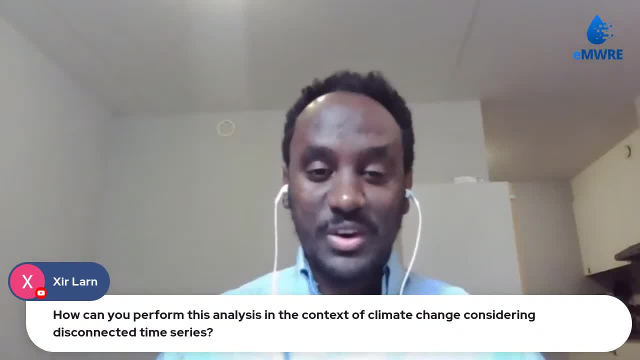 fact, that's uh the uh it. my research currently is all about assessing the impact of climate change on breath. uh, so what you can do is, um, you assess, of course there are different climate change scenarios and the different scenarios that you have- the extreme ones up to 8.5, and then you have the data. so you 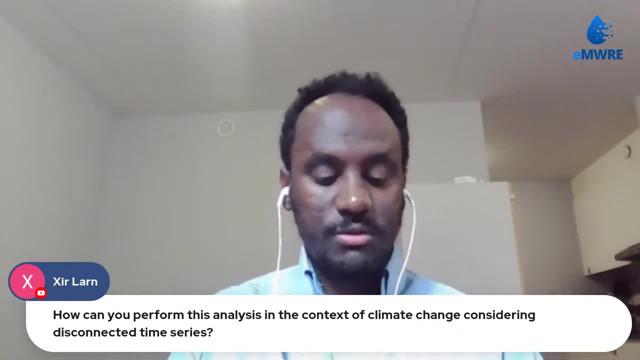 what you do is you calculate for a baseline period, a historical period, let's say 30 years of data. you have spi values and then you have in the future also, let's say, uh, the the last. they say 2070, until the end of 21st century. so you have a very high number of data and then you have a very high 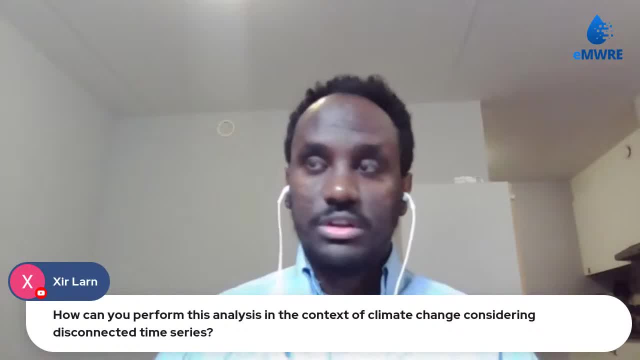 So you compare the SPI values between them and then simple statistics can give you an idea if drought will prevail or not. But recently also we are working on a novel approach where we can assess if the climate signal on the drought can be assessed even beyond just looking into the statistics. 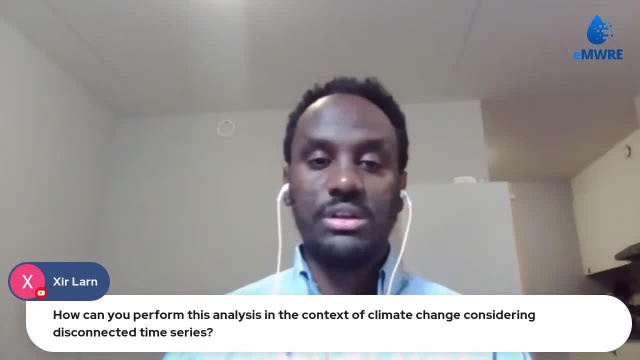 but looking into the severity, the duration and so on and the return period and everything. But if you are interested in that also, I can update you more okay. But that's how you do it: You compare the baseline with the future. 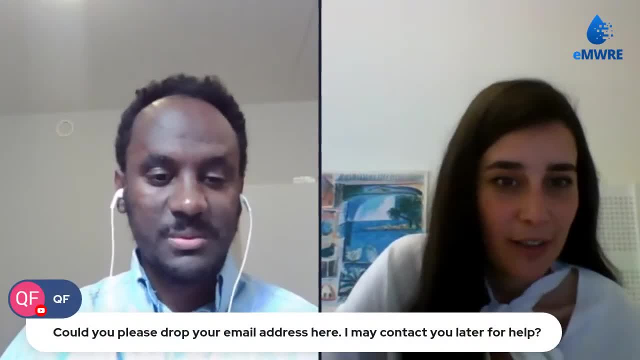 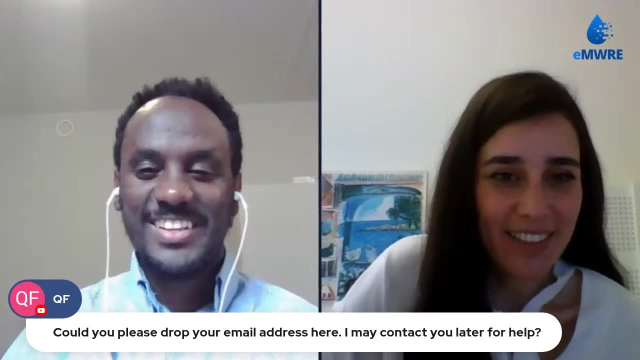 Thank you very much. I think this is very helpful. So I think there are some people interested to ask more detailed questions, So they're asking for the email address. Yes, I mean it's in the presentation, so I will be able to. 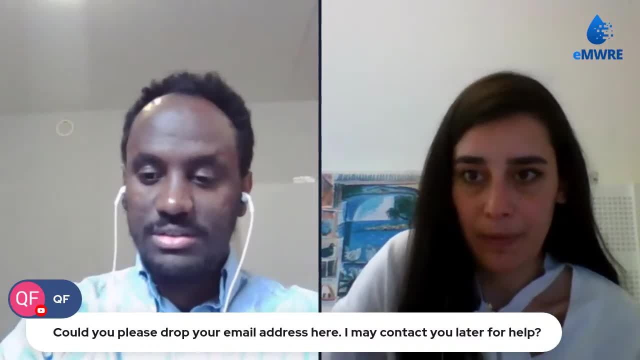 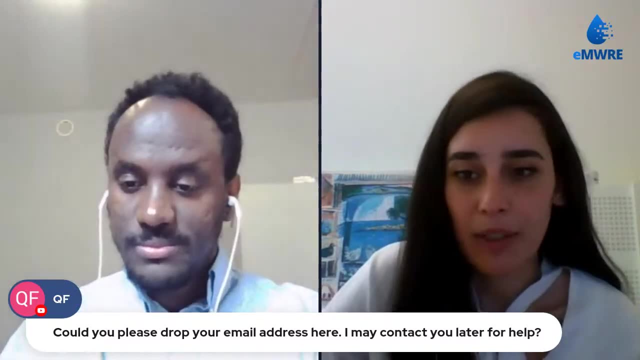 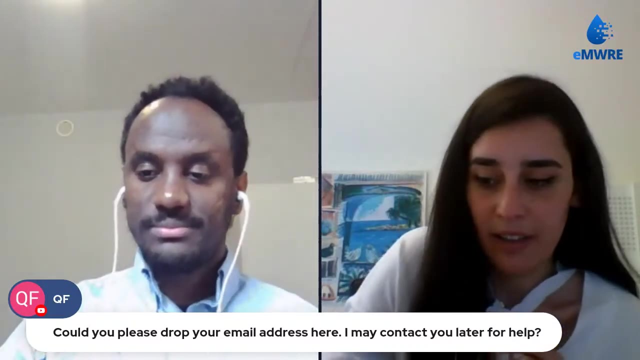 Yes, Okay, Or I can write you here and then you can post it. huh, Okay, So we'll have the email address, But if you have other questions that we can, maybe We still have time for maybe one more question. Yes, 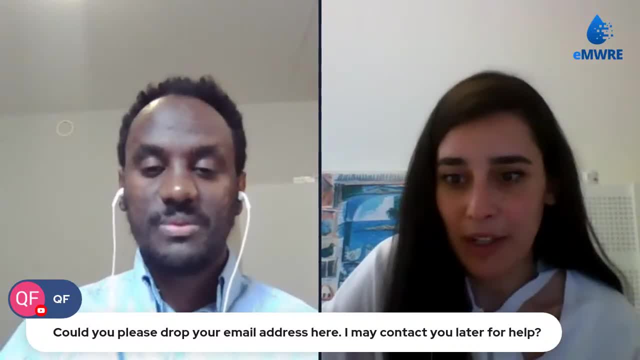 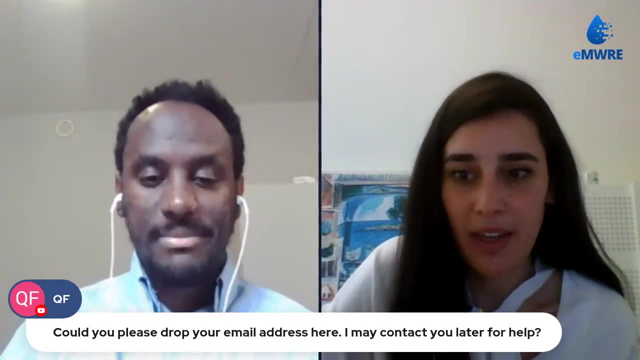 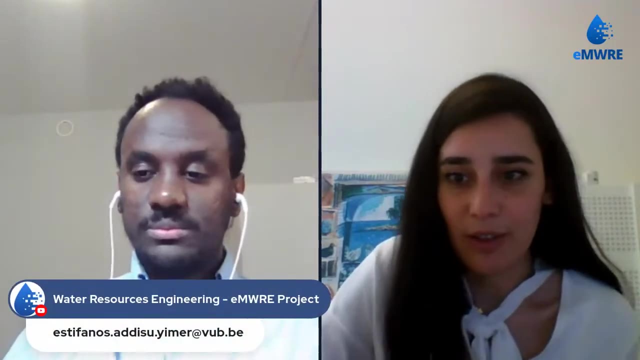 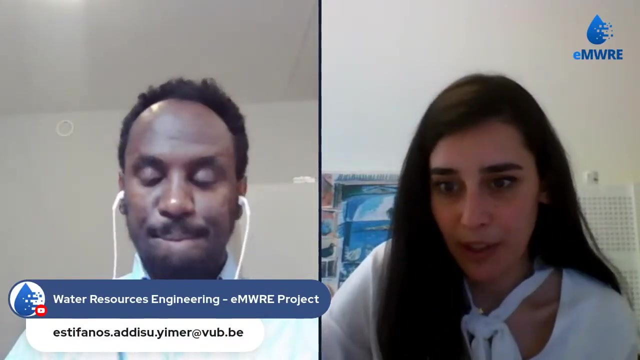 Okay, If not, then you have the email address. It's also in the presentation and the video will be available on YouTube, So also to watch after, And Okay. Okay, I guess we don't have any more questions, but you may be getting some questions via email. 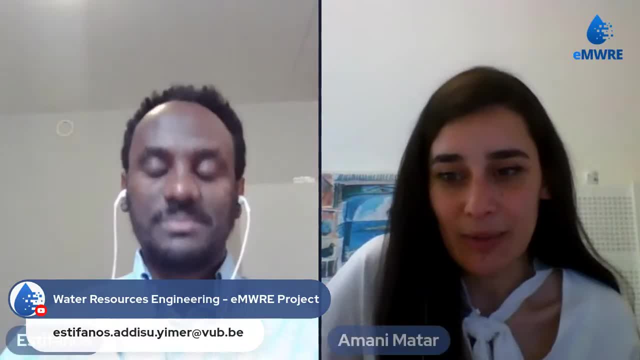 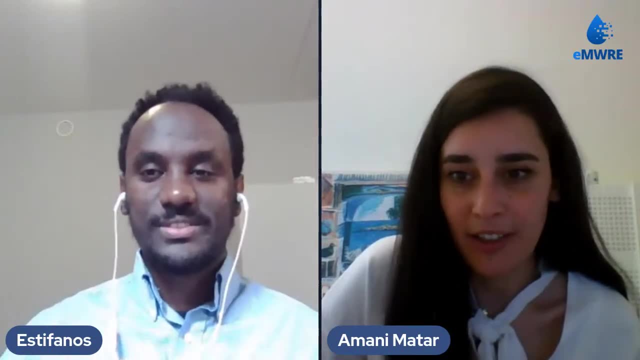 Yes, To answer some of the other questions. Well, I think we can end now. Thank you very much, Stefanos, for being with us And for the very nice presentation, And thank you everyone for being here and for the questions.